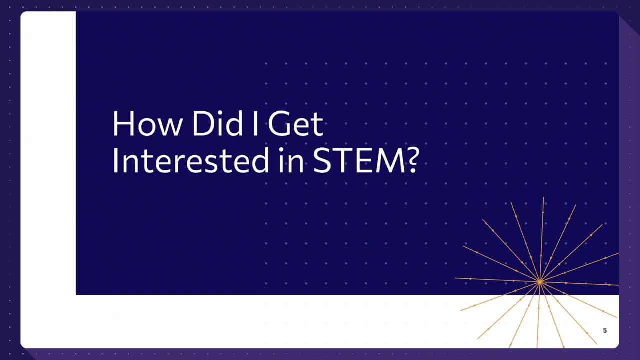 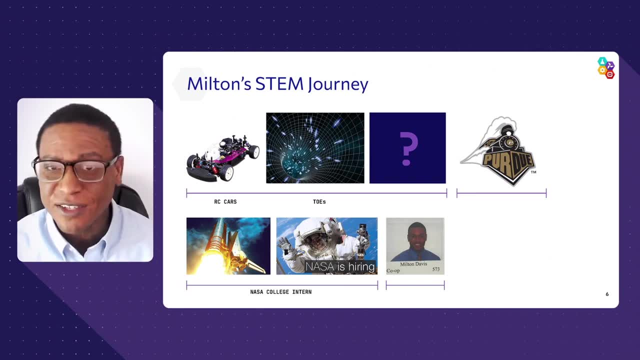 let me tell you a little bit about how I jumped into the STEM field. This is my journey. I absolutely love RC cars. You may have seen this in a previous video. I like to race them up and down the street. I change out the gears, but I'm also really into anything space. Yeah, I have TOEs on there. 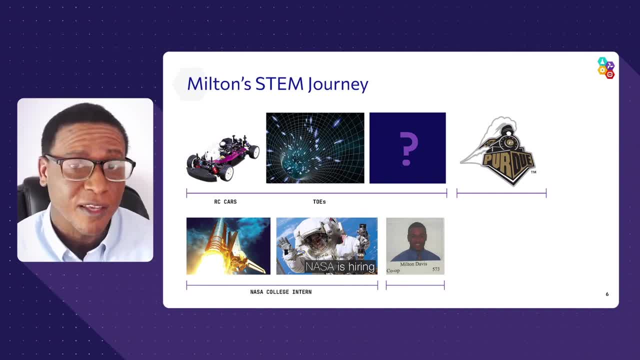 TOEs is not feet, but it is Theories of everything, Like: remember when Matthew McConaughey was an interstellar and he traveled through space and time. He traversed space and time in order to save his family. I just thought that was crazy cool. I debated my physics teachers on Big Bang Theory. 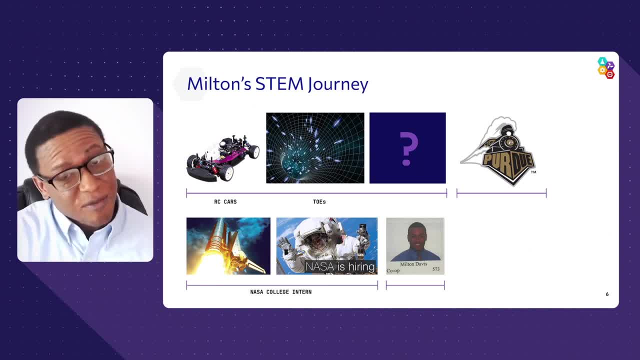 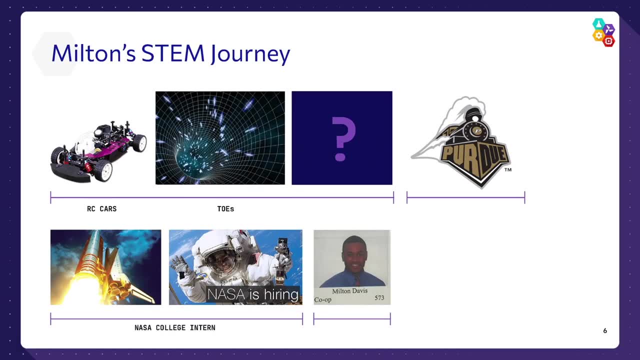 all of that great jazz, But I didn't go to the best school in the world. I say the best technology we had at my school was a typewriter, Great people. but it was a challenge. So I self-rolled a community college And when I was there my counselor said: hey, Milton, you're really kicking butt, but what? 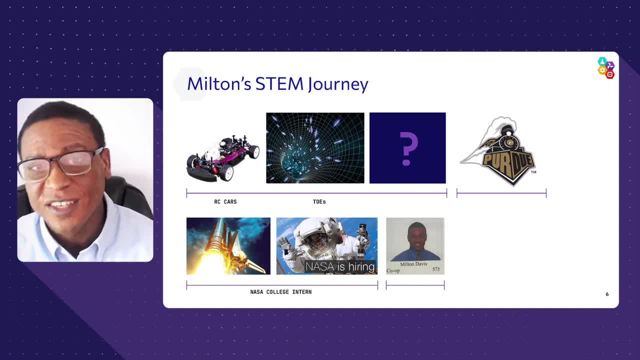 if you're not going to be able to do it. So we mixed all that stuff about RC cars and all those things about space and we landed on aerospace And, luckily for me, he knew some people that would interview me at NASA, And the rest was absolutely history. I've been loving it ever since. 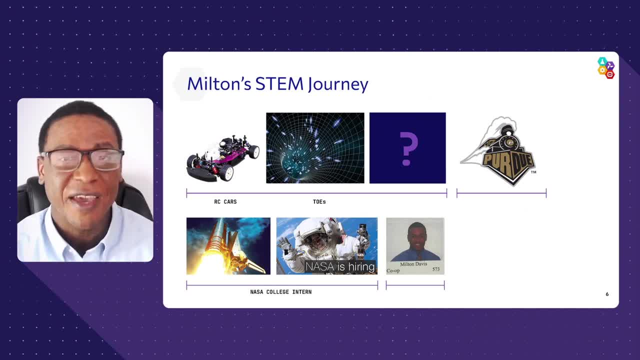 I transferred to Purdue West Lafayette where I got a bachelor's in aerospace and aeronautical engineering. And bam, that is me as an intern a long time ago. But what hasn't changed is we're going to use the same engineering design process that we use on satellites and rockets to develop your space. 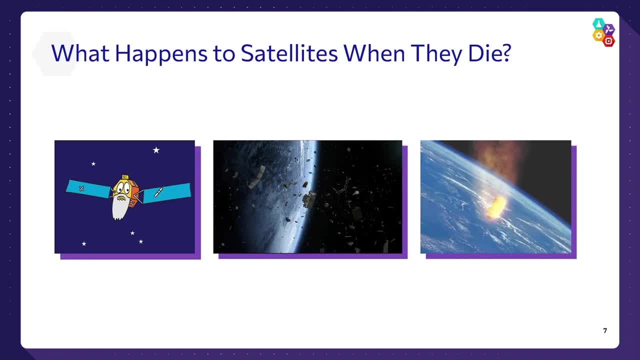 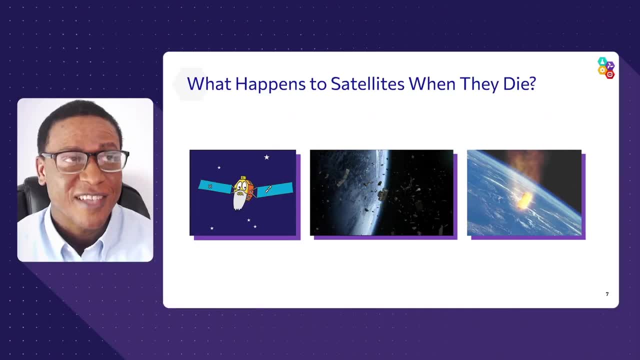 We're going to use our own rocket vehicle today, So I want to talk a little bit about what I do for a living. My main project is helping to address satellites that have died. Do you know what happens to a satellite when it dies? Well, you're looking at top right image. Sometimes it just becomes like 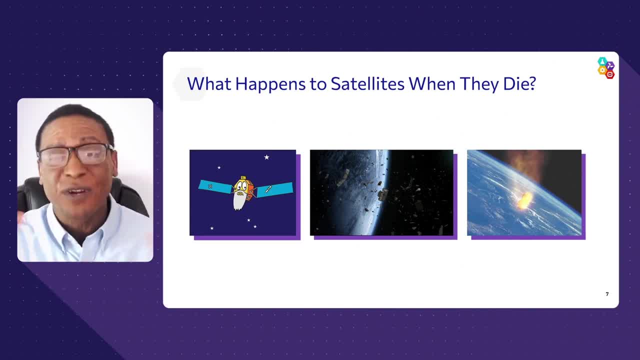 space traffic and space junk And sometimes satellites just collide and run into each other, And sometimes a satellite, you know it may run out of fuel so it can't keep itself propelled. So eventually gravity starts pulling it down And as it pulls it down it's being heated. 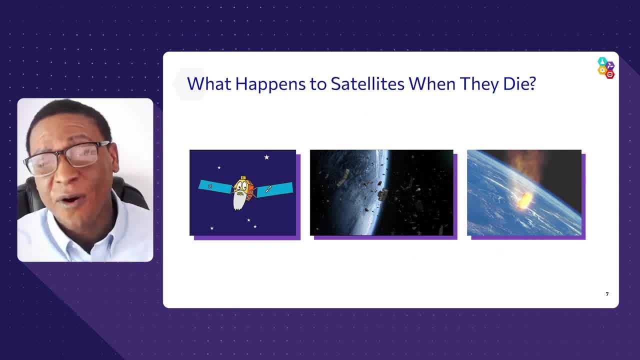 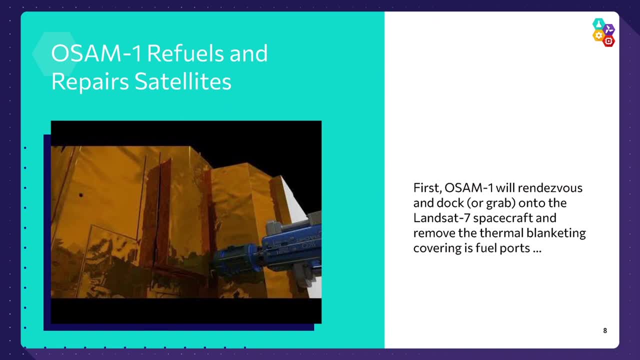 and ablated until it burns up and, hopefully, does not hit the ground right. OSAN 1 stands for On-Orbit Servicing, Assembly and Manufacturing, Mission Number One, And the first thing that we're going to do with OSAN 1 is rendezvous and dock with the Landsat 7 satellite. 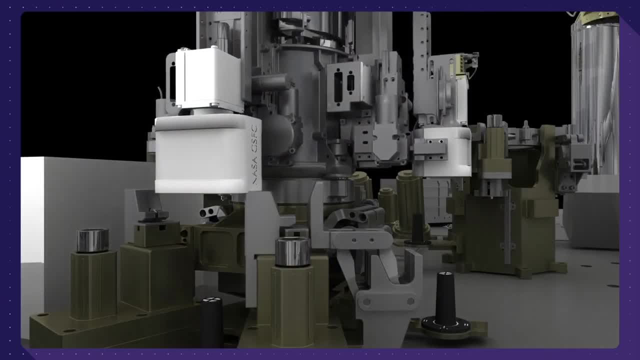 That's a satellite that's been working, but it's starting to degrade, So we're going to grab on to it with a 7-degree-of-freedom robot arm. So we're going to grab onto it with a 7-degree-of-freedom robot arm. 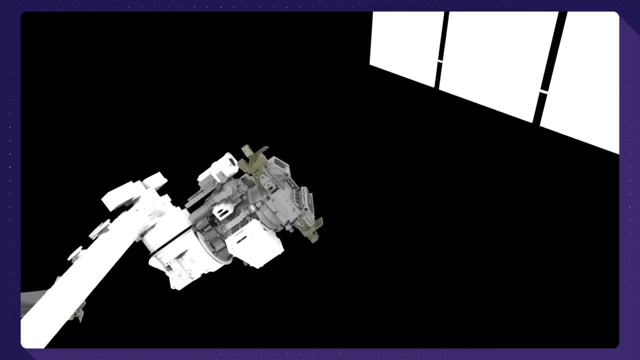 arm. We're going to reel it in, pull it in. We're going to take all our different tools that we have on it. Then we're going to actually cut it open And you'll see, in a minute we'll start cutting. 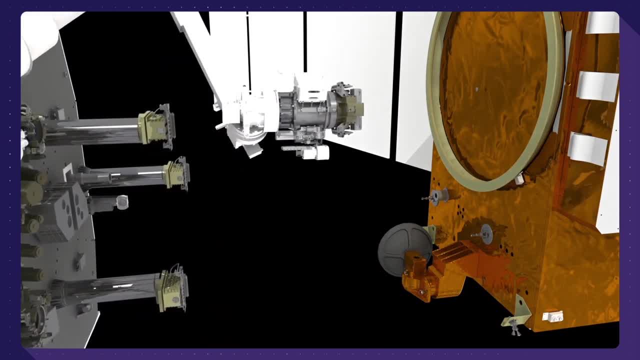 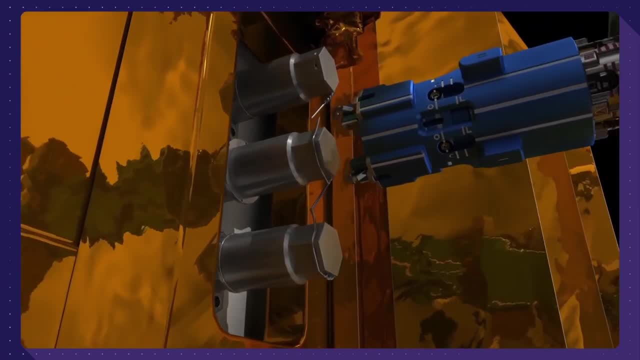 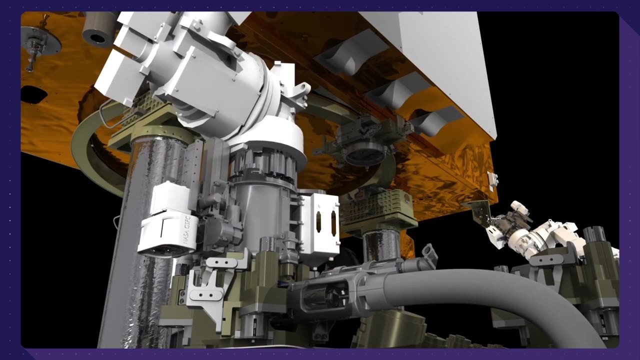 open that satellite And then we're going to refuel it. After we cut open that thermal blanket, then we're going to take the robotic arm and its tool and actually refuel that Landsat 7 mission so we can place it back into its original orbit And it can keep functioning almost as if it. 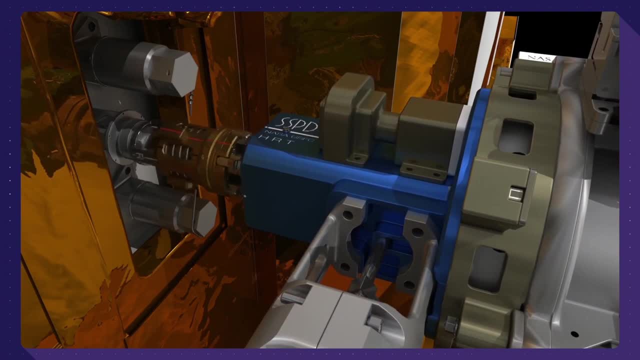 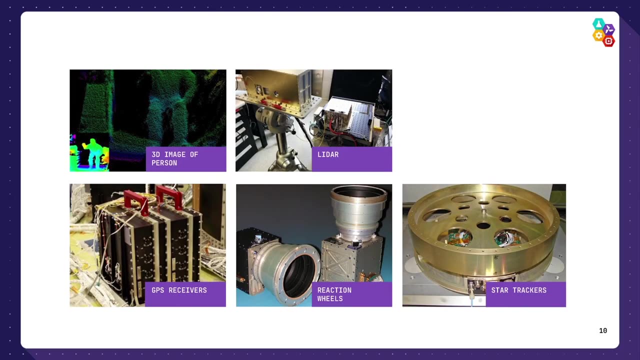 never died. Hey, we're bringing satellites back to life. That's what OSAN 1 is all about. Let me also talk about some different technology that I've helped develop. I've helped develop a LiDAR. A LiDAR is really cool because similar to cars that have sonar and they have self-driving. 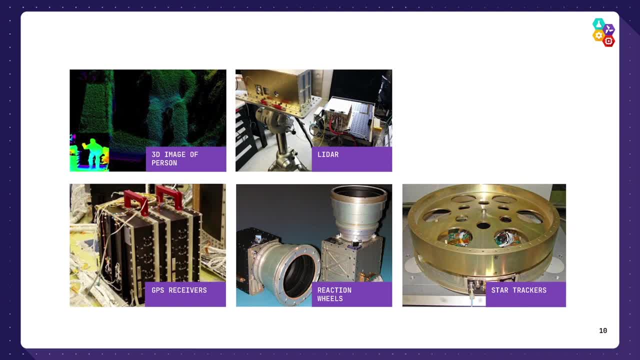 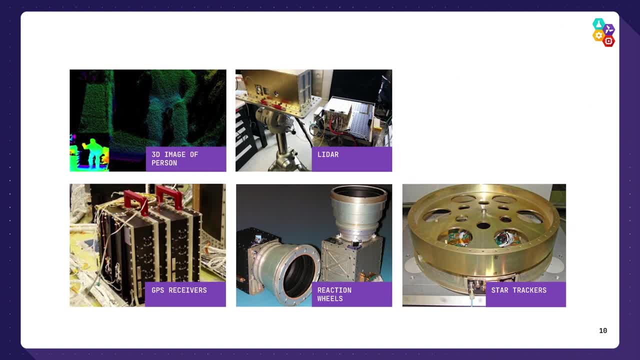 Image of where everything is. So that was a cool product I worked on. Also a GPS receiver. This is a GPS receiver with the world record for the highest orbiting and fastest orbiting satellite in the world And it tells you where you are, Just like your phone. you have GPS right It. 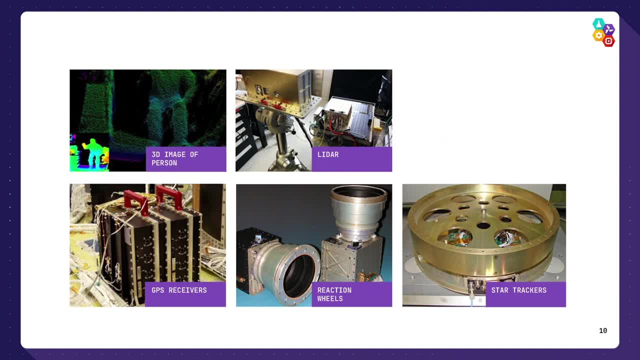 triangulates your position And a reaction wheel helps to rotate the spacecraft so we can orient it And the star trackers tell us exactly where we are. So I've been blessed to work on some really cool missions, But let's talk a little bit about what your questions are. 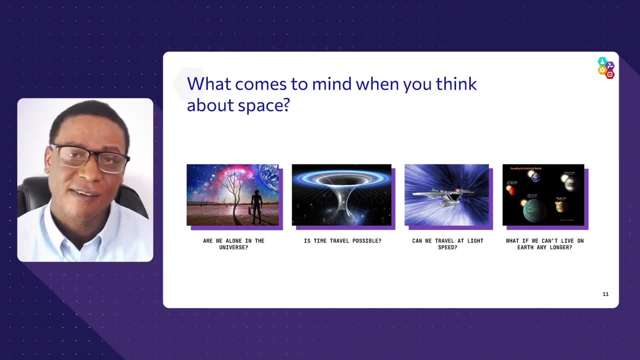 About space. What comes to your mind when you think about space? What questions do you have? What do you think you want to explore? Well, if you're like me, here's some questions I have. I want to know: are we alone in the universe? Yeah, Are there other life forms out there? 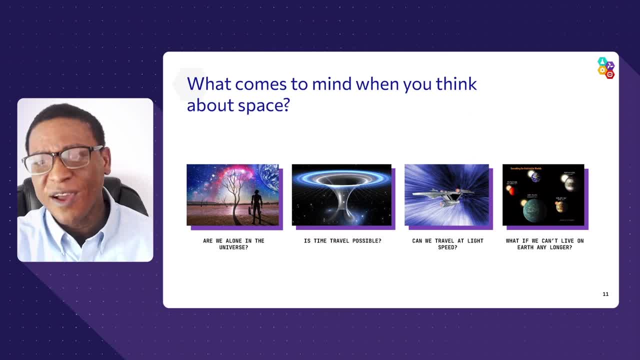 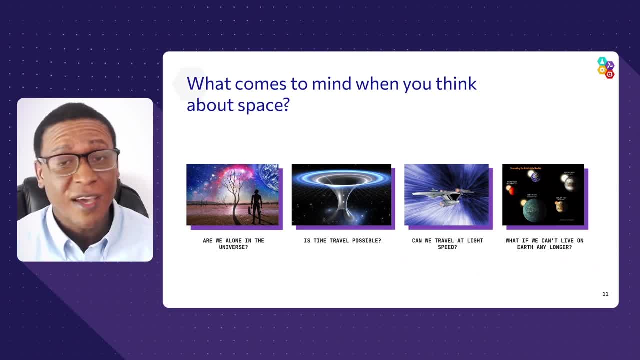 distant galaxies. we got to go beyond the speed of sound. We got to go the speed of light. Can we get there, Or can we travel in time? If we can't travel through time, maybe, maybe we can travel at the speed of light. I'm a huge Star Trek fan, probably even more a Star Wars fan, but I really 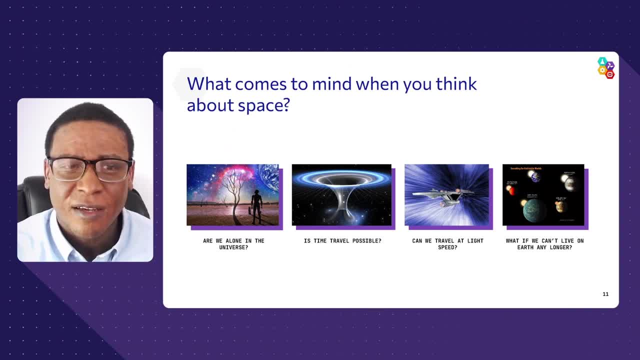 love how they took the time to innovate vehicles that could take us anywhere Across the world. And my last question is: you know what happens if we can't live on this earth anymore? Maybe there's an asteroid coming, like you see in the movies, or maybe we we didn't. 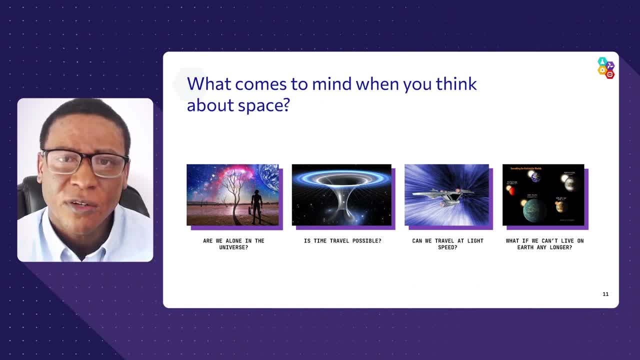 treat our planet as well as we should have. What are we going to do? Are there other planets out there, similar in size, with a reasonable distance from their own sun, that could support oxygen and other things so we can live? Hey, those are the kind of questions I have And I would love to hear. 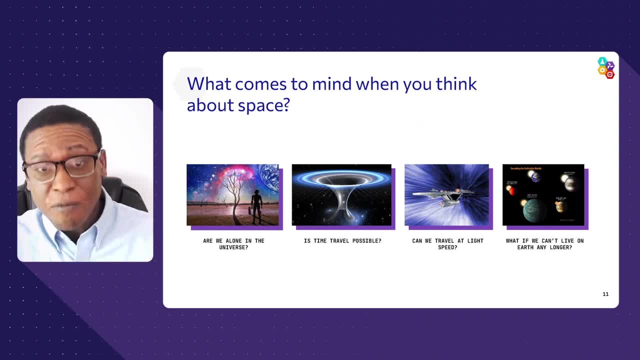 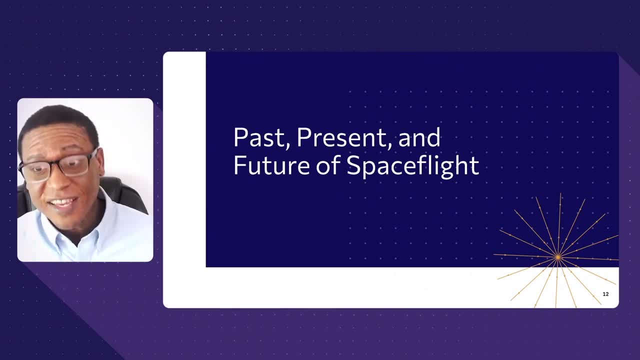 some of the questions you all have. But yeah, this is where we want to go. Let's talk about the past, Like how did we get here? And then we can talk a little about the present, And then after that we can talk a little bit more about you all and how you're going to take us to the future. 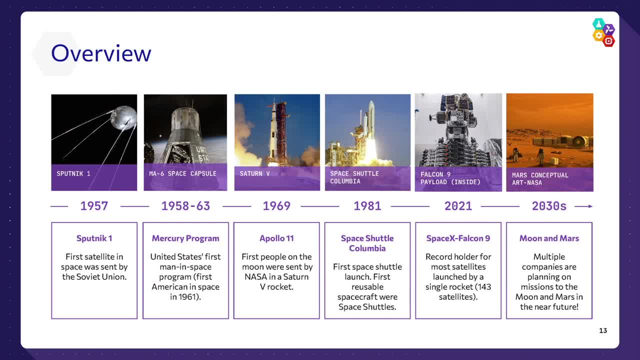 So how did it all start for us? Well, there was a huge race to get into space, And actually the Soviet Union was the first one to get a vehicle into space. That was Sputnik 1.. And as soon as they got a vehicle, 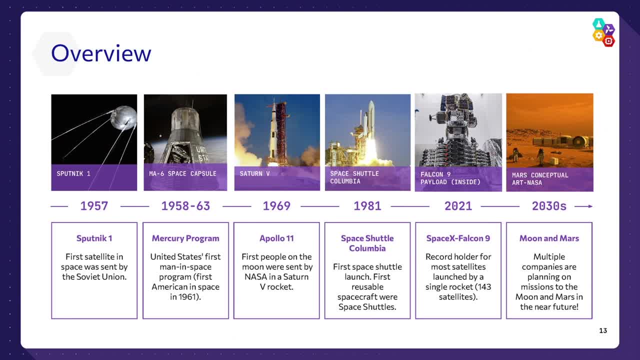 the space. you know the Americans say, oh, we got to get in the game too. The MA6 space capsule- that's from the Mercury program- was able to place the first American in space And then following that, you know, we had all those different Apollo missions and we're trying to get many humans into. 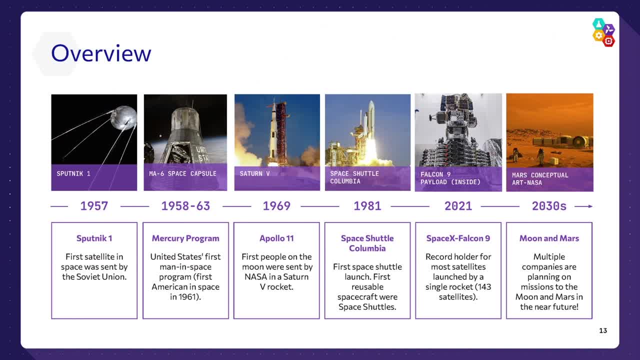 space. But we realized we got to get better rockets. If we're going to launch into space, we got to get better rockets. So we started with the Saturn V, which was taking multiple people in the space at a time- A couple, a year. But you know, we realized that to really investigate space we need to have 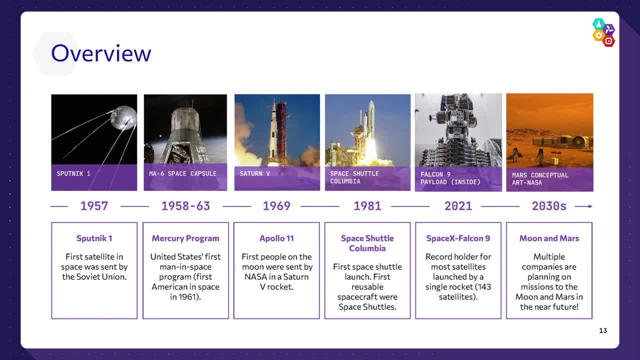 multiple people going into space at multiple times. So the space shuttles started And the space shuttles were really, really great because they allowed us to have somewhat of a reusable portion of the shuttle itself, But most of the rocket that was expendable And the rockets are. 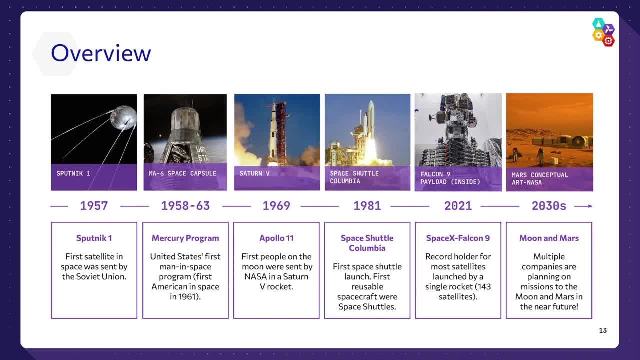 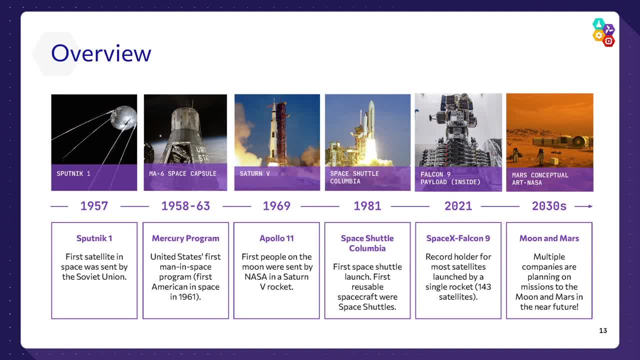 And they can innovate. And you've seen it. SpaceX has done something that is unbelievable: Developed a rocket that not only can launch into space, it actually navigates almost autonomously to land on the ground, And that portion that's laying on the ground is. 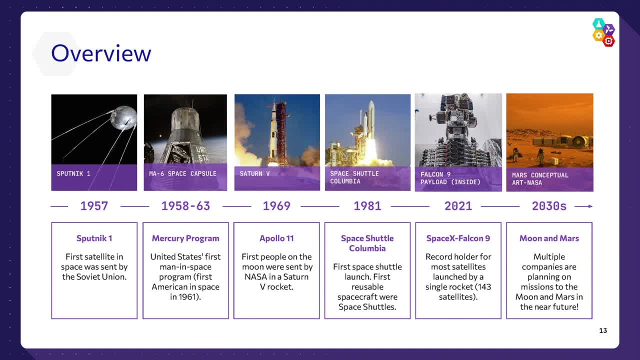 reusable. So now we can have reusable shuttles, We can have, in some regards, reusable launch vehicles. I mean, we're just kicking butt, But none of this compares to what you all are going to do, Some things that you're going to do, like live on Mars. 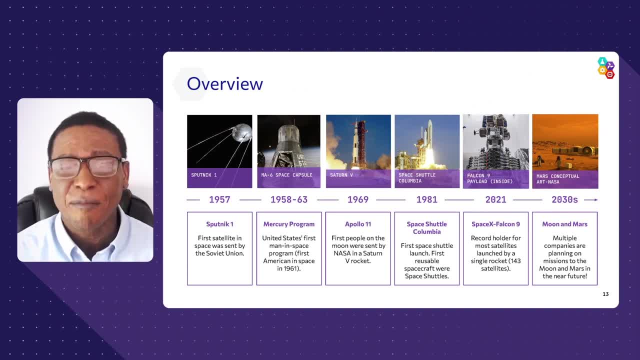 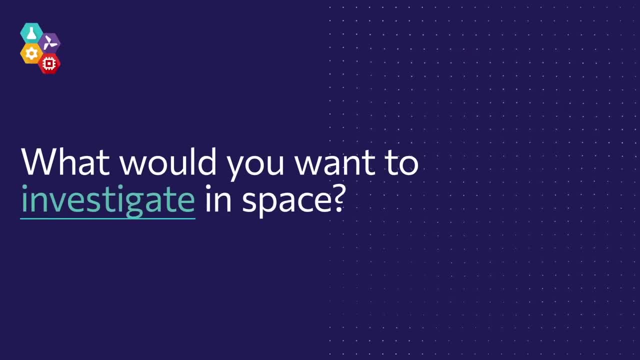 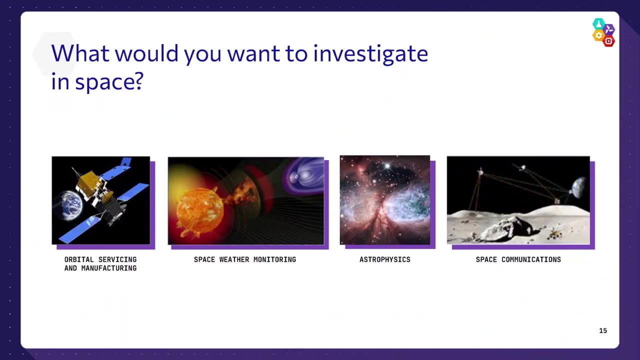 I mean, in your time, it's going to be absolutely unbelievable. So that's my next question for you: What would you want to investigate in space? What are some theories you have, What are some things that you want to find? Would you want to travel into space? Man, all that stuff is just so. 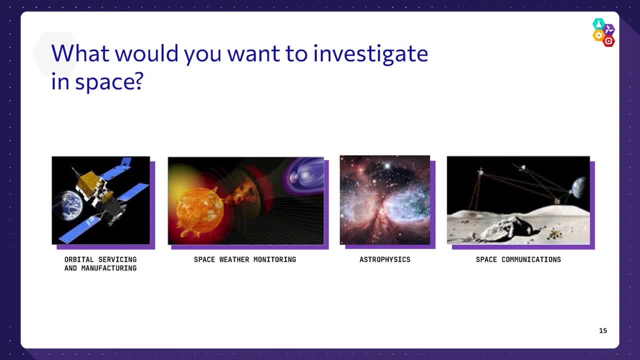 so crazy cool. Let's talk about some of the missions and how they're organized. First, space communication is pretty important. Why? Because if we can't communicate with things like the rover on Mars, then we can't reorient it, We can't get images, We can't get video, We can't. 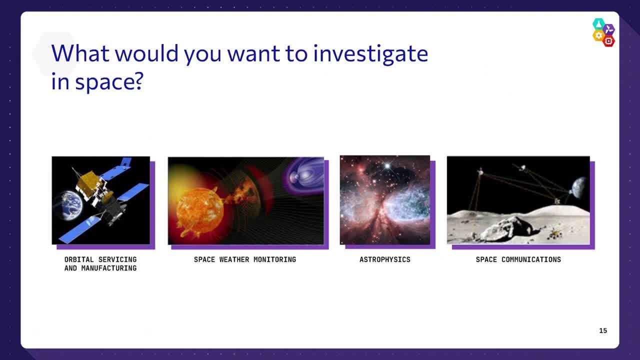 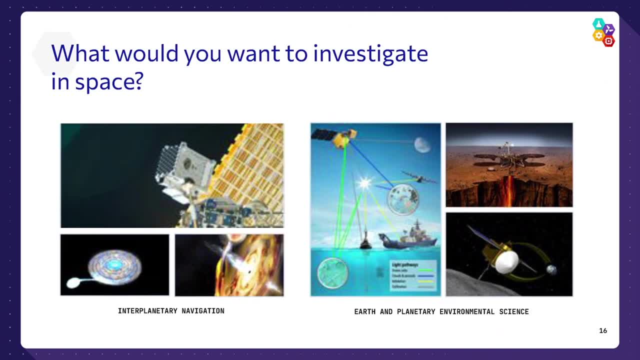 see what's going on in real, almost in real time. So space communication is important. And then we have to navigate. you know interplanetary navigation. How do we navigate between different satellites? How do we navigate between different planets? How do we navigate from the Earth to the? 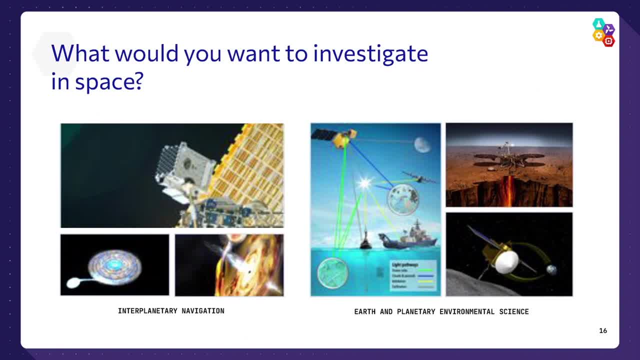 Moon to Mars- All that is extremely important- And Earth and planetary environmental science. Now you may be thinking, man, that's a lot, But we have to protect our Earth. We're living here. We're going to be living here for a long. 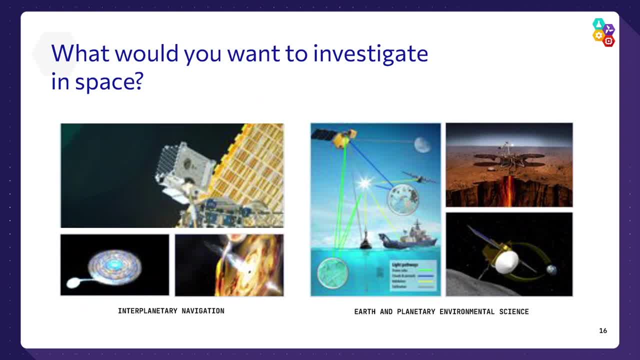 time, When hurricanes come around, when storms come around, we use satellites to help predict what's going to happen, so that in the end, people can get out of that area in a reasonable amount of time. All of that comes through that environmental science. Then there's the orbital servicing and 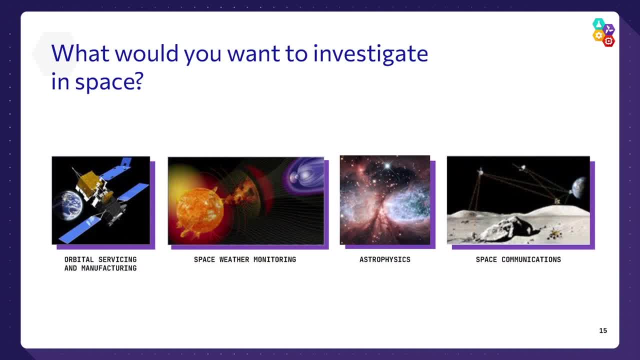 assembly. We talked about that. We're going to fix some satellites in space. There's some space weather monitoring. You know, the sun puts out those crazy solar spurs that could do some damage to our Earth. So we're always investigating that. And if you're like me and you 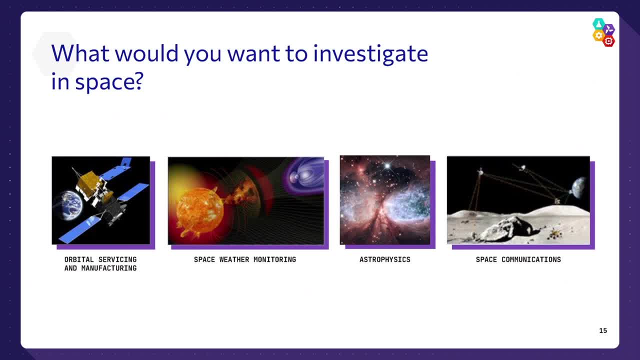 want to learn about aliens, you want to learn about distant planets, then you are all about astrophysics. So that's the main components of the types of mission as we perform in space. But here's another question for you: What do we send in space? What are all the different types of? 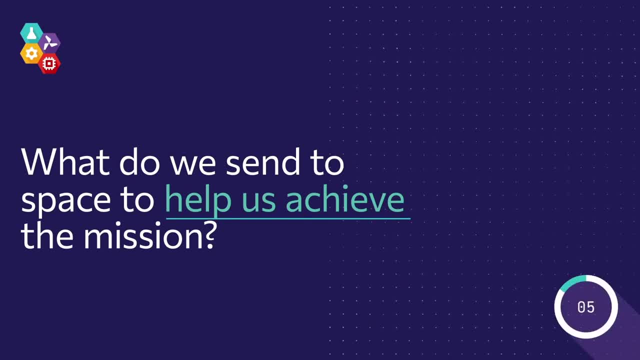 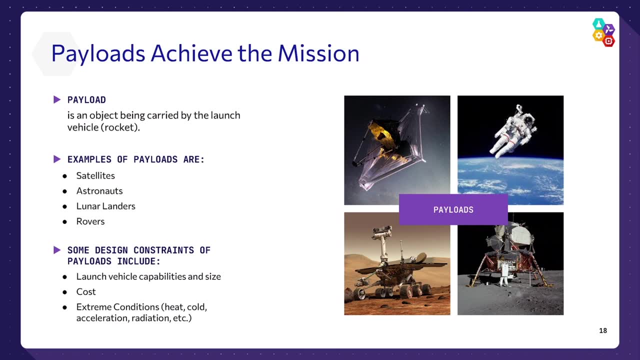 things that we see in the space and how do we classify them? Yeah, it's payloads that achieve the mission. Payloads are what we send into space, And a payload could be almost anything. It could be a satellite, It could be you, the next astronaut, It could be the lunar lander, It could be a rover. 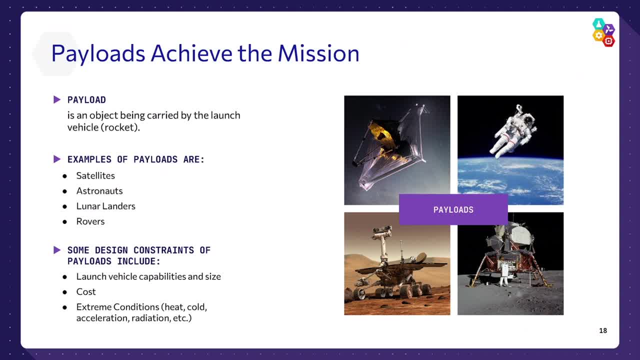 that's on Mars. Anything that we send into space is a payload. Here's some examples You ever heard of the James Webb Space Telescope That's just investigating everything that has to do with history of our universe- Astronauts for sure, And this Mars rover which we talked about. 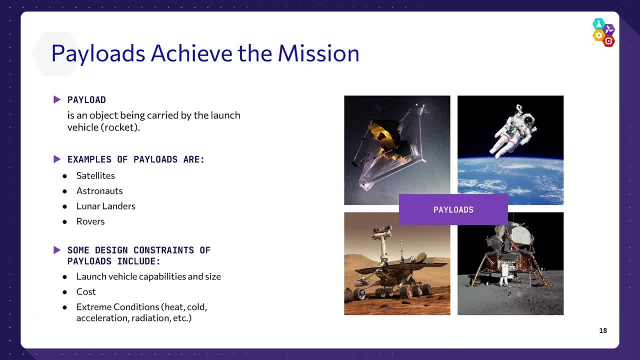 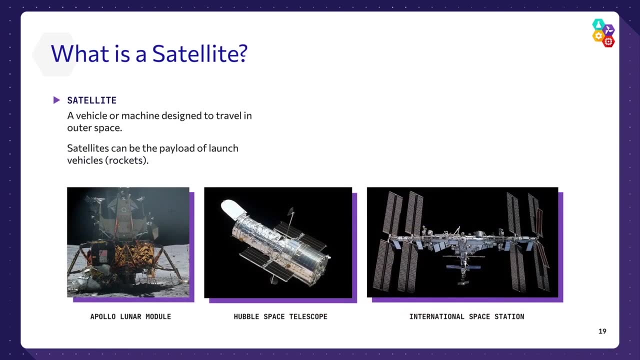 that's a payload, Yeah, And anything that we send on the moon, that's a payload. These payloads have to be designed to survive some very extreme conditions too. We'll talk about that later. But the main thing that we focus on for most of our investigations are satellites- Satellites that may dock with. 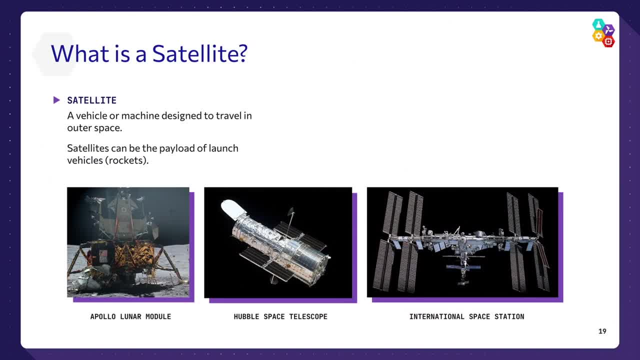 the International Space Station or a satellite that is performing different missions that could be in our future, light years away from our Earth. The satellite is what's placed on the rocket that is sent into space, And that's what we send into space And that's what we focus on for most of our 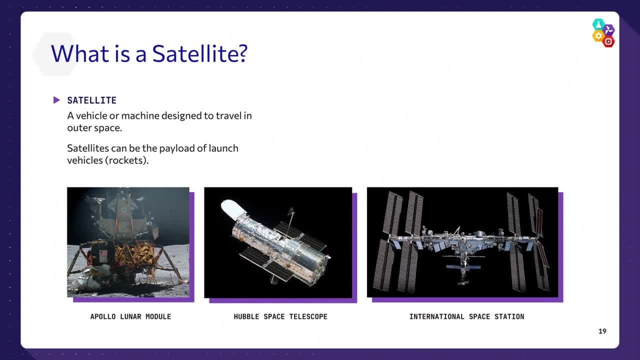 space experiments And we constantly have this narrative that when we do this kind of thing, we just don't do any of those things, We just don't have access to the satellites, any of the available satellites that we are getting into space to perform these. 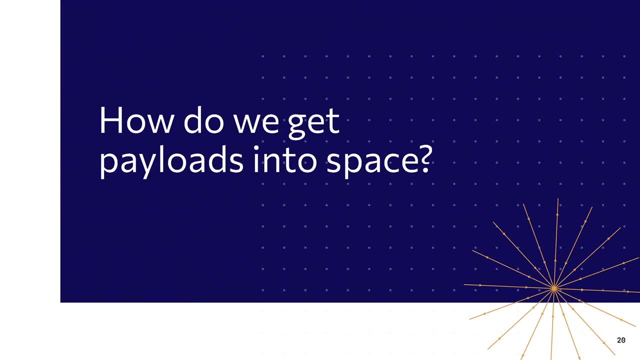 different investigations. So now we've got our satellites, We understand those. How do we get the payloads into space? This is big. How do we get the payloads into space? We have to stylishly ask ourselves to integrate our satellites into space. What do we use? 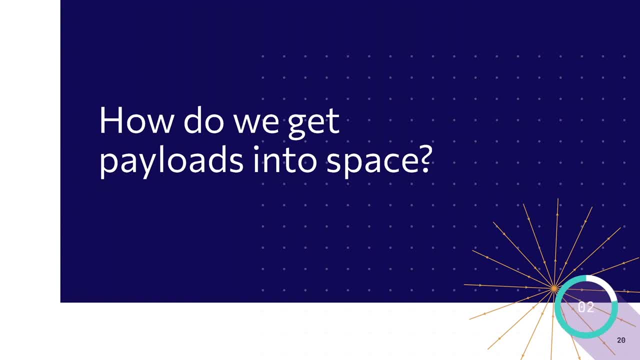 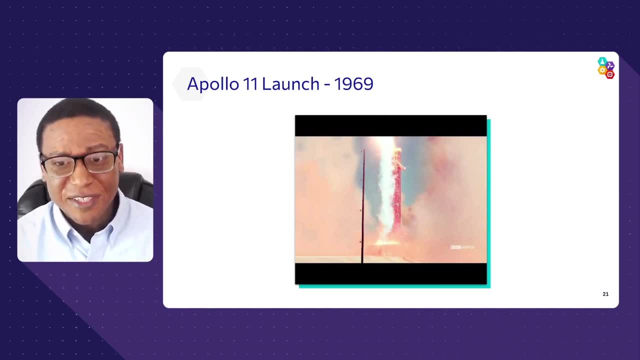 Big, Strangest Words. Well, if you said rockets, you are correct. It is rockets. that's how we travel into space And, as I will put it this way, I have a really, really nice video to show you about a rocket that. 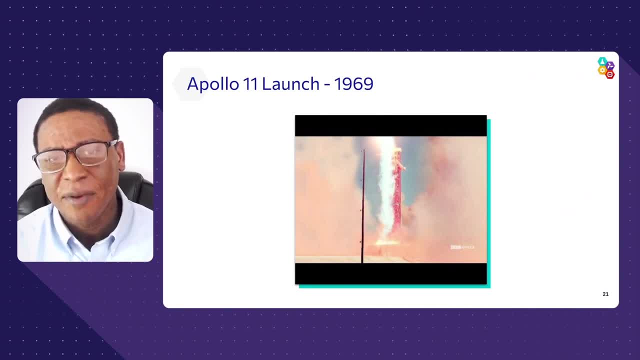 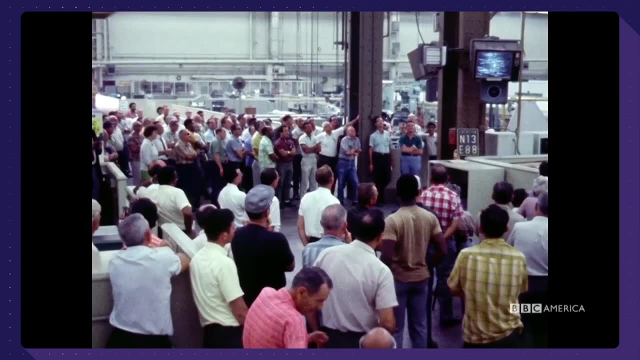 was backuisagged or maybe they just haven't been shipped on recently. We'll talk about that in just a minute, about a rocket that was pivotal in our time: the apollo 11 launch. that launched some of the first people all the way to the moon. internal 12, 11, 10, 9. ignition sequence start. 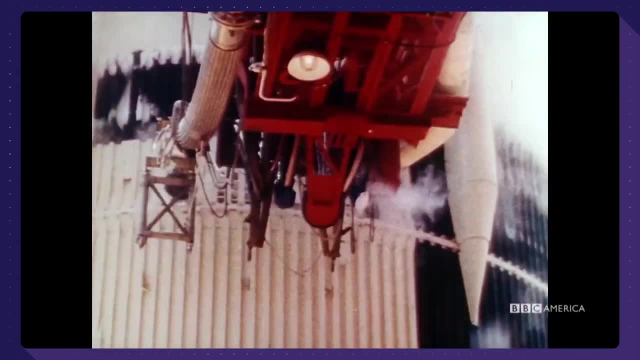 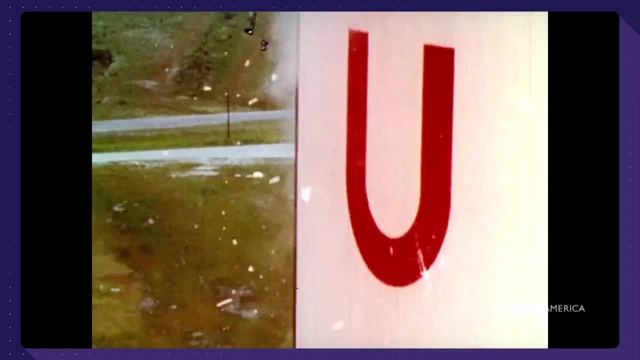 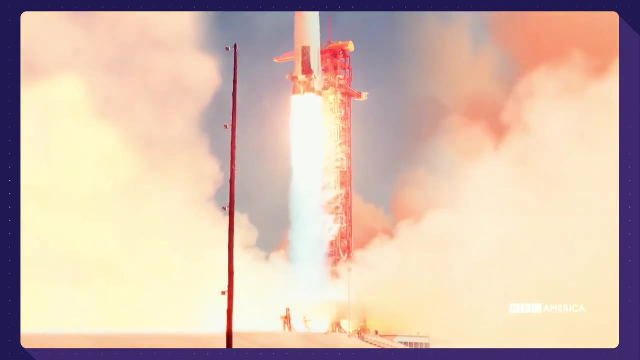 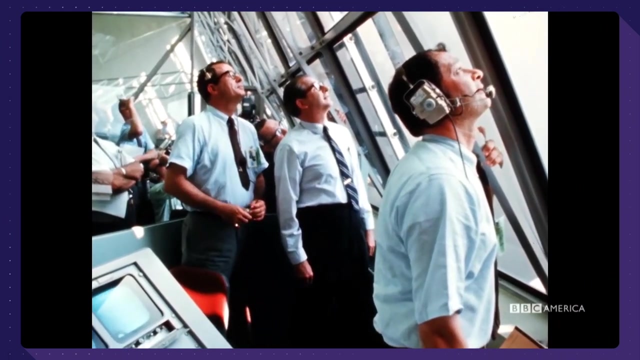 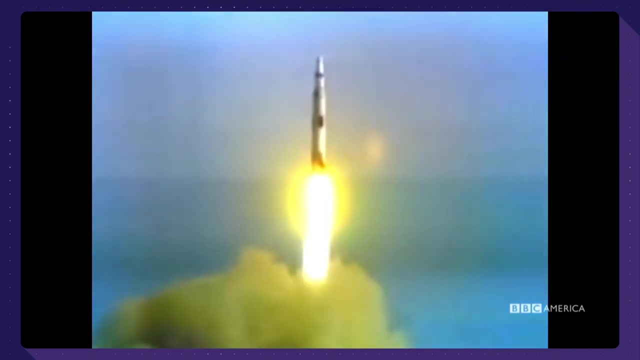 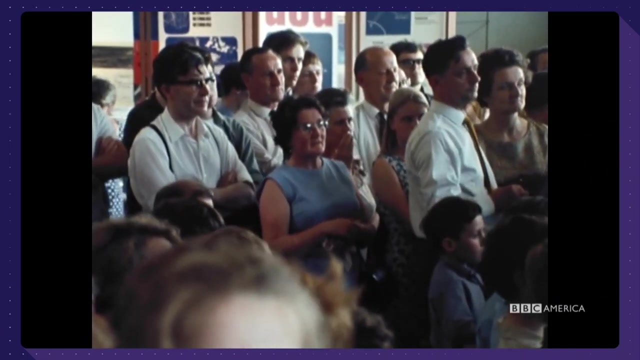 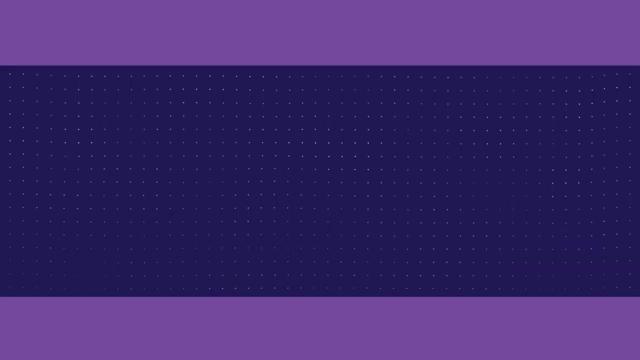 all engine running. lift off: we have a liftoff 32 minutes past the hour. lift off on apollo 11. tower. do we have a roll program 30 seconds? wasn't that video just awesome? i mean you could see the people's faces. i mean unlike you, i mean. 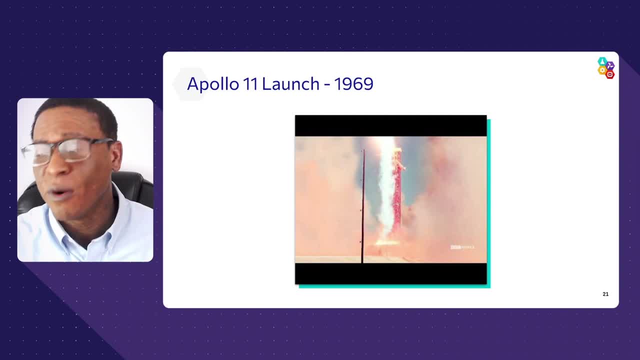 you've seen spacex, you've seen people you know multiple times- astronauts from different countries in space, but this is the first time in our country, in our world, that we really have seen someone travel to the moon. they were absolutely in awe of this moment and again we're going to be in awe. 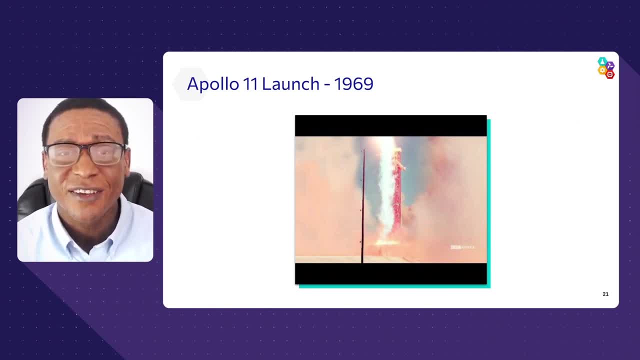 of what you all do in your time. i mean, you're going to take it, you're going to take space and space travel just to the next level, for sure, but first, before we, before we go to that next level, how do we get there? well, first we have an atmosphere. right, the atmosphere we got to. 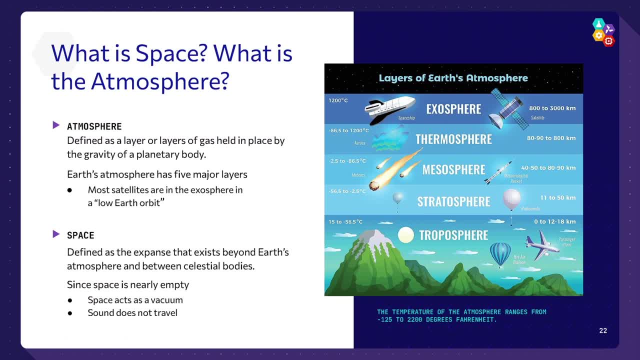 travel through that before we even get into space. now the atmosphere is a lot of air and molecules that uh could cause drag and it makes it difficult for us to. in addition, with gravity, makes it difficult for us to get into space. right, but the atmosphere is important, it's very important, did? 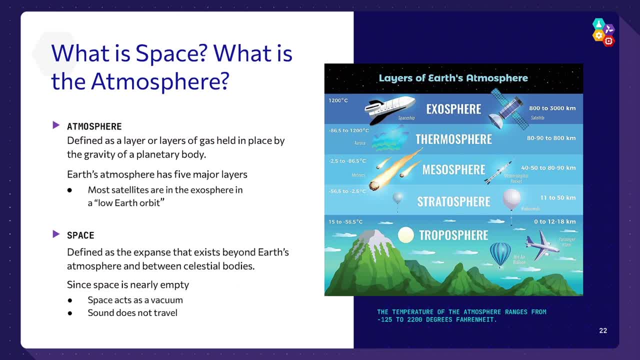 you know that it's almost like a blanket covering the earth that keeps us in a reasonable temperature so that we all can survive without our atmosphere. with something like the magneto sphere, the solar radiation would hit this earth and we probably wouldn't have life. we think that mars at some point lost its atmosphere, lost its magnetosphere. 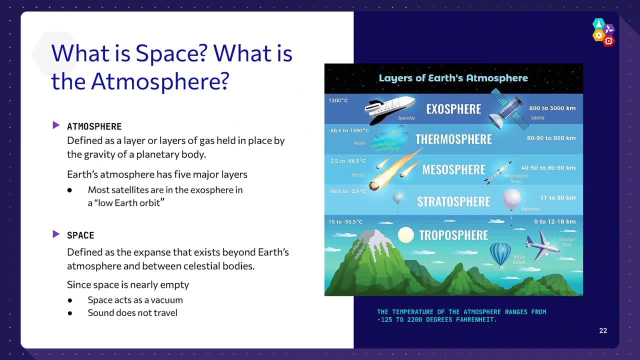 and that's why it can't support life. so the atmosphere is extremely important, but, yeah, there's a lot of forces that we have to fight in the atmosphere in order to just get into space, right, and then, once we're in space, you know we're not protected by that atmosphere anymore. 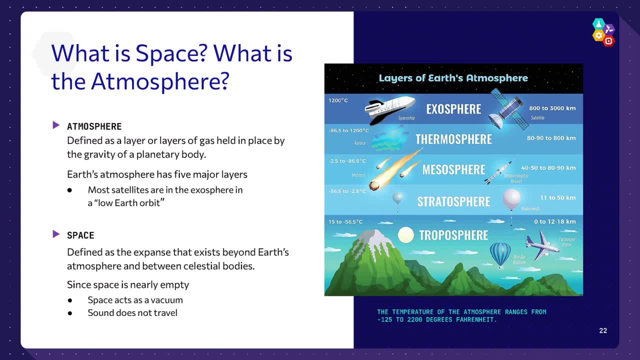 so your rocket, your satellite, has to be designed to survive some extreme temperatures. it has to survive this vacuum in space. sometimes your satellite will be shadowed or behind the earth. it can't see the sun, so it's extremely cold. sometimes it'll be right in front of the earth, looking directly at the sun, so it'll be extremely hot. 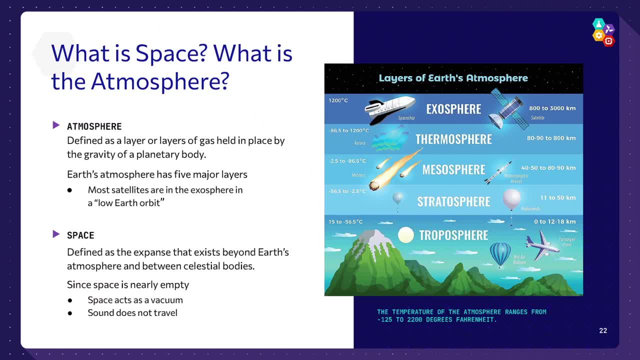 all the electronics, all the structure, it has to survive. and there's radiation going on, it has to survive electromagnetic interference, all these different things going on. they have to be designed to survive all of that once we're in space, right, and so that's why we have to survive. 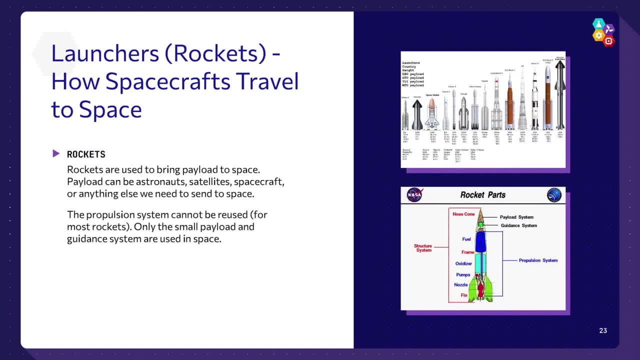 in space. so now we talked about space and what we have to travel through in the atmosphere. what do we use again to get into space? well, that is the rocket right, and this is what you're going to develop: a rocket. and you've seen that the game here is. you know, satellites get larger and larger. 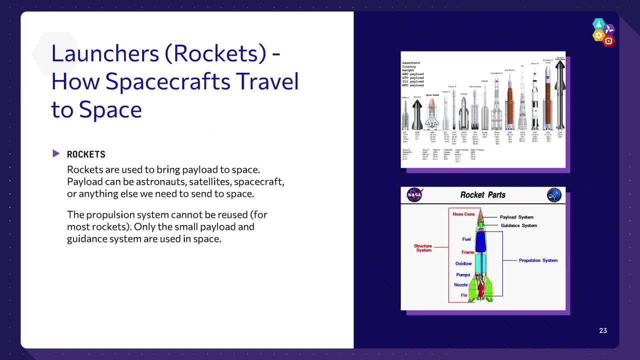 the james webb space telescope spans almost the length of a football field. they're getting larger and larger. so rockets have gotten larger and larger and larger, for sure, i mean, we got to get more and more stuff in the space of. rockets have just gotten crazier and crazier and crazier and 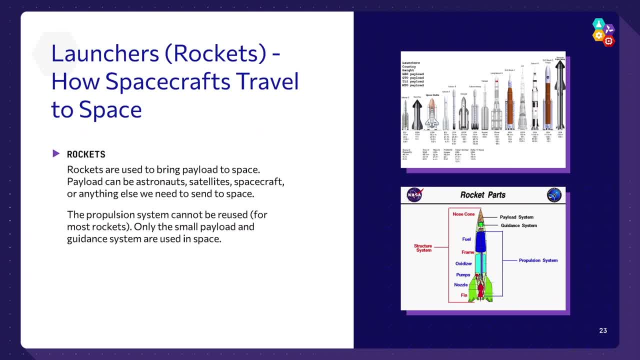 crazy large. um, they carry the astronauts, they carry the satellites, they carry other things that fix satellites. i mean we're just all over the place with what we put in the space. but look at the rocket parts. when you look at the rocket parts, i mean you see the fuel, the frame, the oxidizers. you 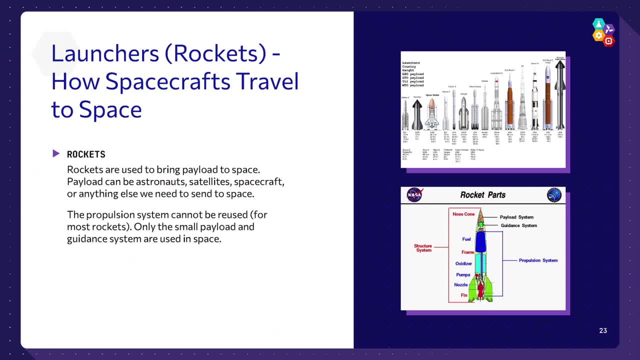 see the pumps- that's all important- and the fans and the structure, but at the top is the payload. when you look at this, it's very interesting. the payload is only 10 percent of this entire vehicle. that doesn't seem efficient, does it? it's not? i mean at this point this technique of using rockets and then and the efficiency that 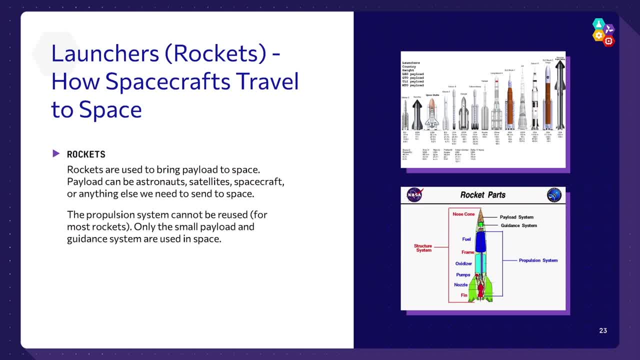 they have. we only get a little bit of payload that we can send into space and we want you to help improve that and that's why we're giving you a really, really cool project and maybe we can improve that through our propulsion system. maybe we can improve that through lightweight new 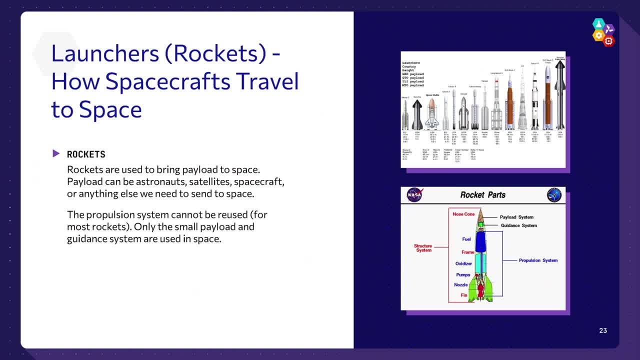 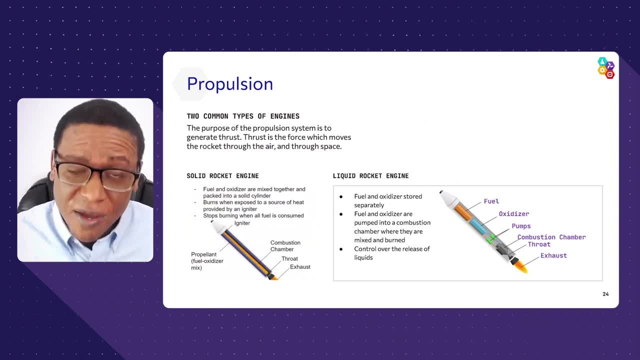 materials. we'll have you think about that when you develop your rocket. but let's talk about propulsion a little bit. there are two different fuels that we use and systems that we're going to use to propel rockets into space. the first one is the solid rocket engine and the solid rocket engine. 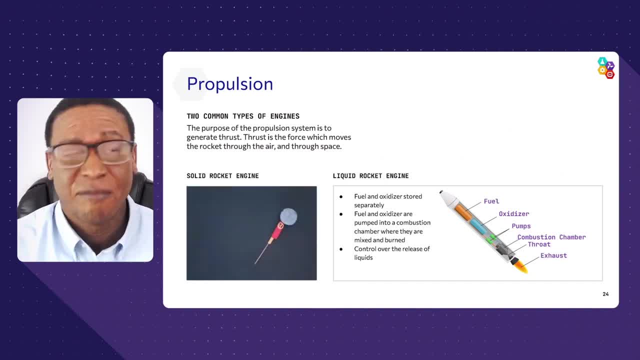 is almost like your bottle cap now. when i was young, me and my brother used to have these little rocket bottle cap things that we would launch at each other. that's dangerous. we probably should have done that, but it's very similar. what you learn is, once you launch it and you let it go, it's powerful. 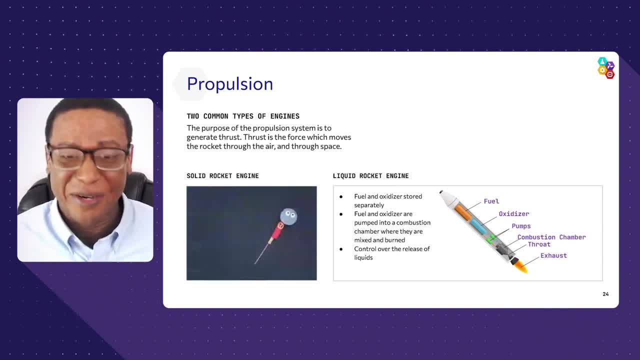 it's fast, but there's no control in it, there's no stopping it right. that's how solid rocket engines work. there's, there's no control in them once you launch it. it's gone now versus a liquid rocket engine. now, a liquid rocket engine is different. you do have some control, you do have some throttle. 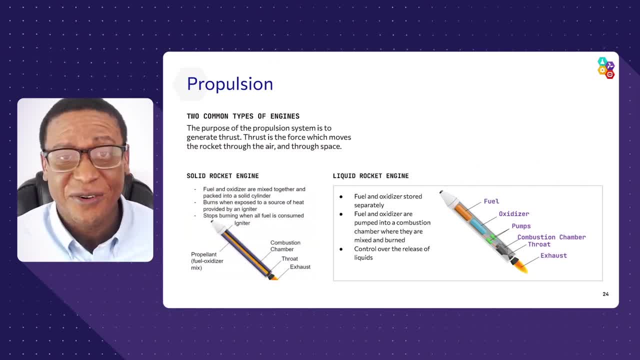 it's almost. you're sitting in your car. you hit the gas, you go, you go forward, you want to give it a little more gas. you go faster, you give it less, you decelerate right, you let go of the gas. hopefully you slow it out and stop. it's very similar with a liquid rocket engine, maybe not as powerful, but it. 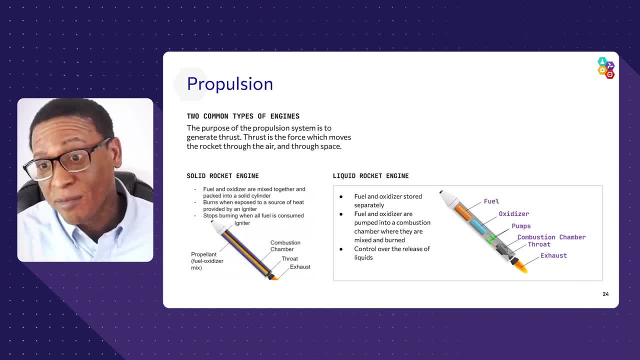 gives you that control, and we need both options, sometimes and within a rocket, in order to achieve what we need to achieve. so now you have, you understand satellites. you understand spacecraft, which are payloads. now you understand the launch vehicles, which are the rockets. it's time, finally, for you to develop your own rocket system, and that's your. 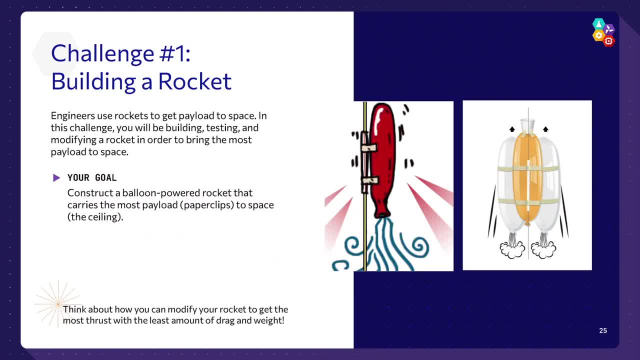 challenge here today. challenge number one is to develop your own rocket and it's going to launch a payload in the space. you're going to build it, you're going to test it, you're going to improve it. all that great jazz. we've given you a lot of information and we're going to give you a lot of. 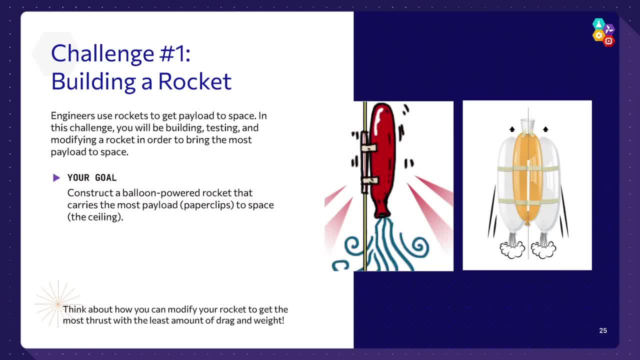 information, and we're going to give you a lot of information, and we're going to give you a bunch of different balloons and other things in your kit and what we want you to do is tape a part of your line or your reel to the ground and then see how much mass and how quickly you can launch that. 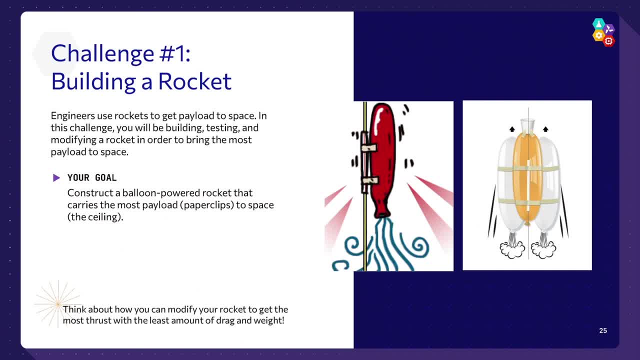 rocket all the way to the silver. that's your goal. hey, maybe you start with no mass, start a little easy right and then slowly start adding mass until you get to the point where you absolutely can get anything in a space. and maybe you take some of those great ideas, you implement it and help folks. 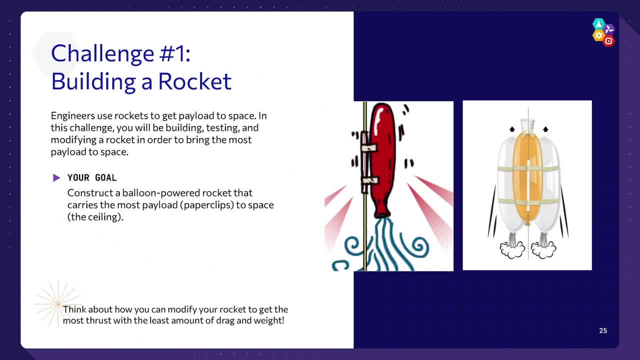 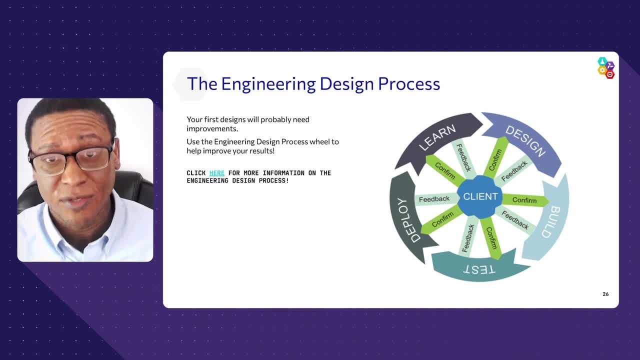 develop even better rockets. that would be really, really cool. but what we want you to use for your tool to improve is the engineering design process. okay, so before we just start throwing those balloons and straws and fishing line all together, do a little research on rockets. do a little. 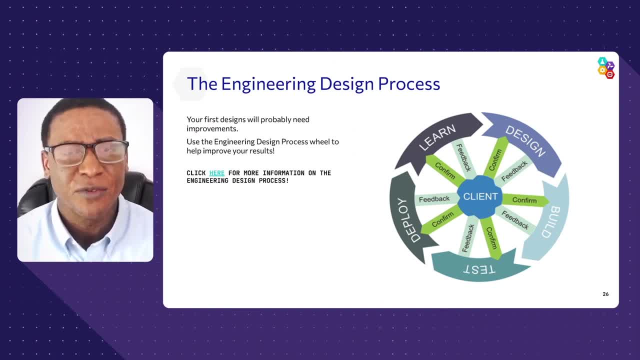 research on rocket balloons. what are some of the challenges you have to overcome when you have to develop them and then make a design? once you make a design, you draw it all out, you map it all out. trust me, when it's time to actually build it, you're going to build it and you're going to. 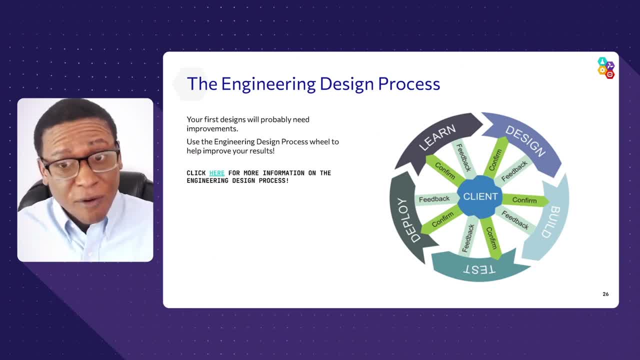 build an even better product. then, after you build, don't be afraid to fail, test it out. see what, what issues that you have that, uh, maybe you got to discard or maybe you need to improve to make the rocket even better. we've given you multiple balloons. we've given you a lot of tape. you've 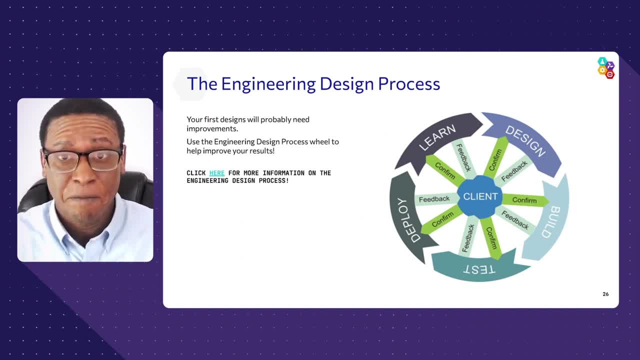 got a lot of materials, so you can keep doing this over and over and over again. now, me personally, i have been blessed to obtain a couple patents. every one of the patents, these innovations that i've obtained, have come through my failures- not through my failures, but through my work, and 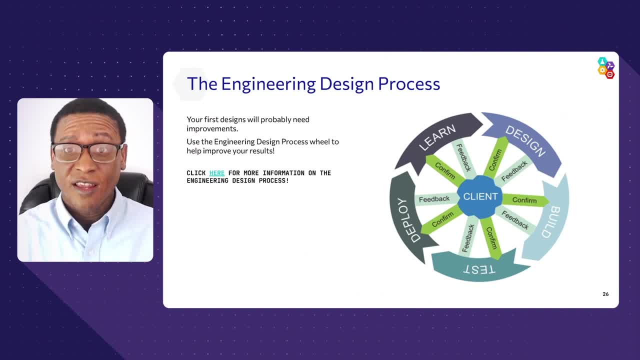 through anything that was easy and then, after you have something that's great and that's working, now it's time to deploy it. maybe you all have a rocket competition in your class. i can't wait to see it. but as you're thinking about this, are there already some ideas that you have floating around? 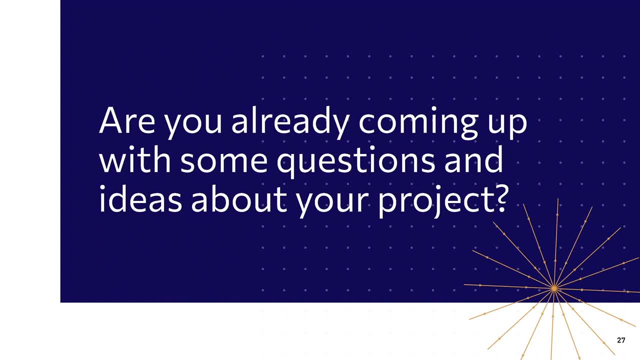 your mind how you're going to make this a really, really cool, a really fast, a really powerful rocket. maybe there are some questions that you have already. you can spend a little time to just start jotting that stuff down now. the more you think about it, the more you research, the more you you plan, trust you're going to have a. 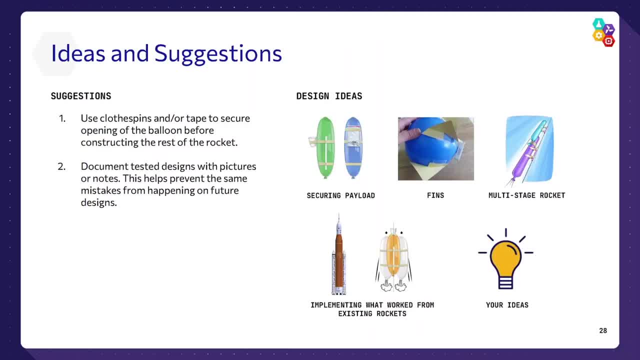 much better product. we also have some ideas and suggestions for you, some ways to kind of get your mind thinking about this rocket. how are you going to attach the straw to the balloons? how are you going to keep them secure? think about friction. how do we reduce friction? how do we ensure that? 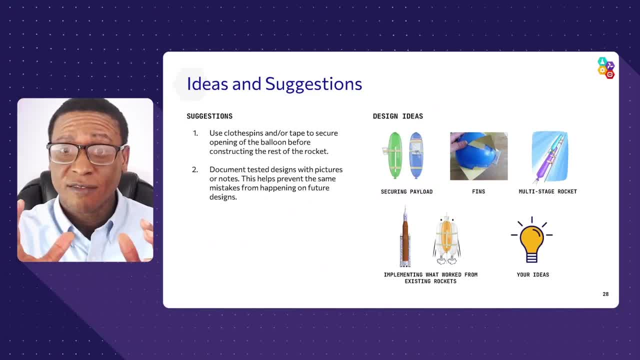 the rocket, when it's traveling up, stays straight. so if you want it to stay straight and navigate in a way that is straight from the ground to the top of the rocket, you're going to have to add some fins to control some of that lateral movement, to control some of the spinning maybe. 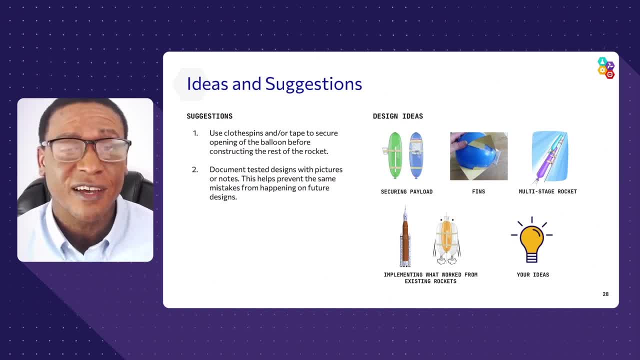 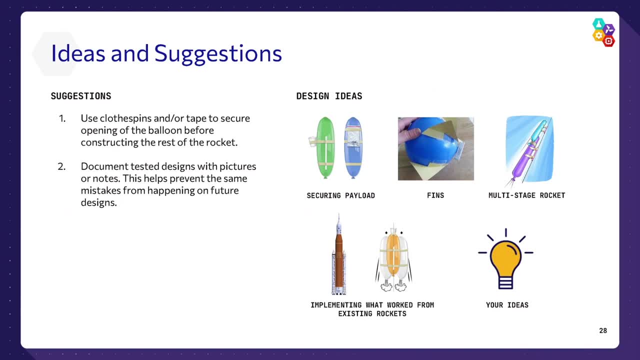 when you added a rocket, you don't think it has enough power to get you all the way to the top. it just kind of goes to the middle, midway and then it stops. think about staging, that staging is where you have multiple rockets. the first stage gets you from the ground to some level, then the next. 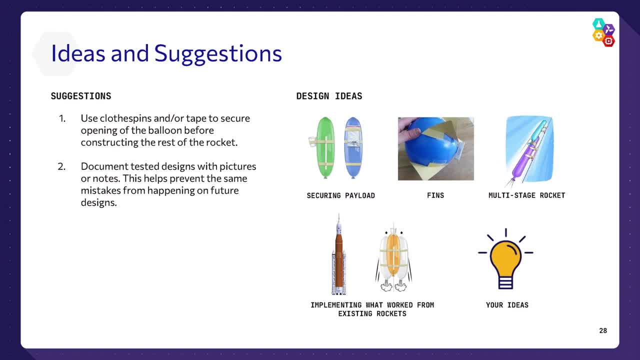 stage is, take you even further until you get out of the atmosphere. maybe you could come up with a cool way to stage also. you know, you may think i'm just going to add a bunch of different things to the different rockets all at one time and just have full power, full thrust, full throttle until i get. 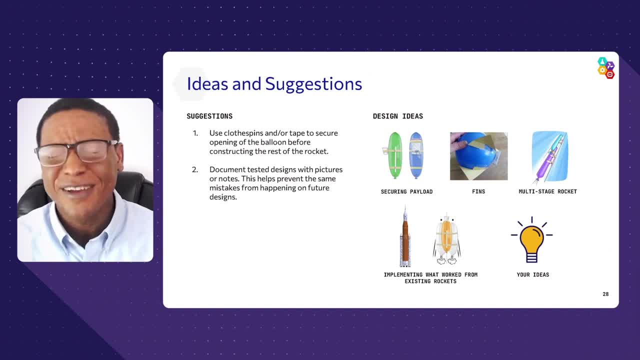 into outer space. hey, any ideas you have, try them out, test them out. as long as you're trying, you're good to go. okay, here's some other suggestions we have. you know, try to use a clothespin or tape to secure the opening to the balloon. you know, because you want an easy way to keep trying this. 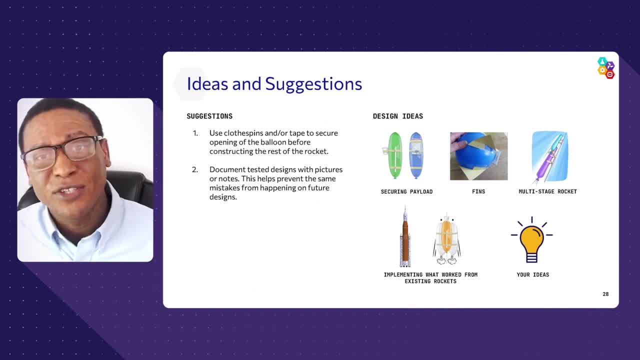 over and over again. you want to have an easy way to release that pressure from out of the balloon. and then we always want you to document your design, because in this engineering design process you may try this 10 times, but maybe you think, man, i need to go back to number three. so as long as you, 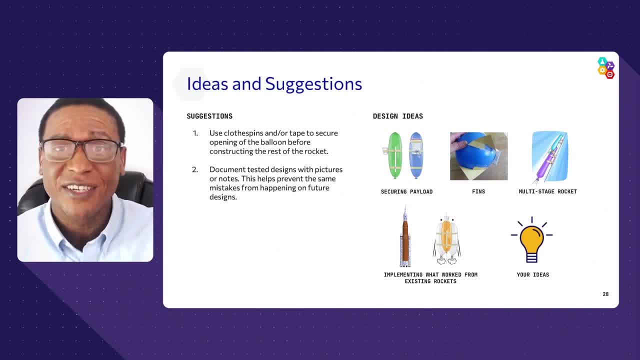 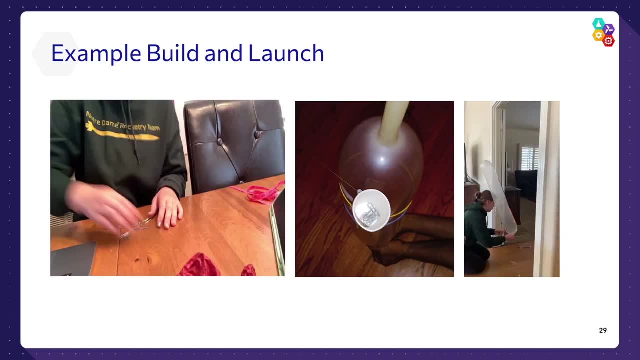 documented that. hey, number three had boom, boom, boom, these different ideas. you go back to it, you improve that one and that may be the best one. let me show you some pictures as well. this is a short video that kind of goes through katie, one of our engineers, building up her rocket and, as you're, 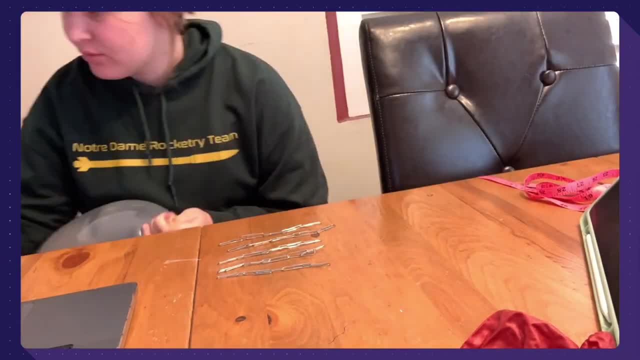 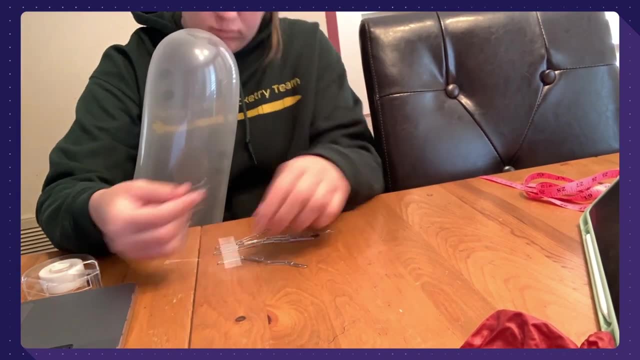 working through the process, come up with some good techniques to secure the straw. come up with some techniques, like we said to- to hold the end of the balloon closed. think about maybe using multiple straws in order to secure a very, very large balloon right. there's a lot of different ways that you can. 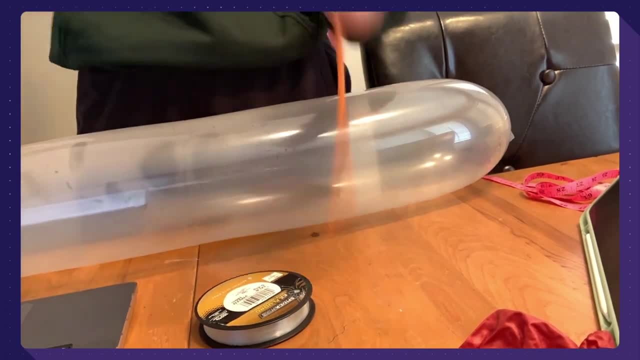 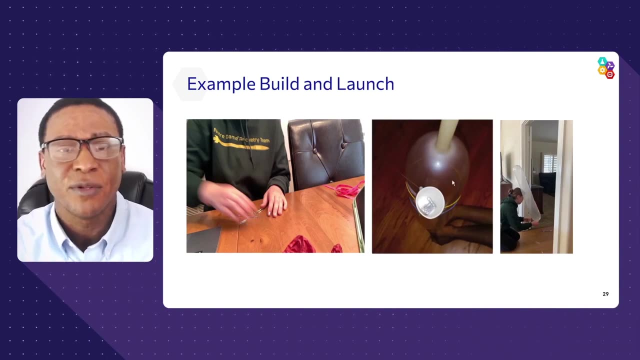 think about solving this problem. oh man, katie, you're absolutely killing it. look at that. and also, i'm showing you just an image of how to place this cup onto your rocket balloon. now, this cup is kind of secured directly to a straw. that's an idea i came up with. hey, you may come up with an, even. 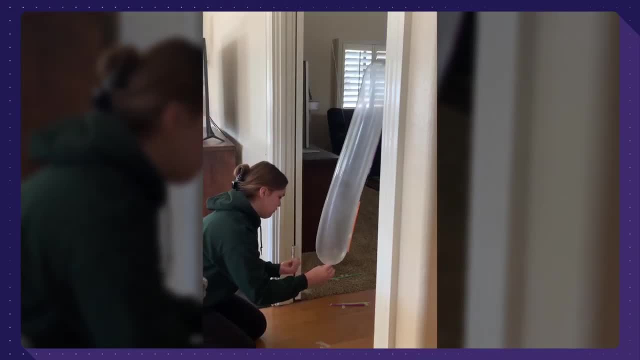 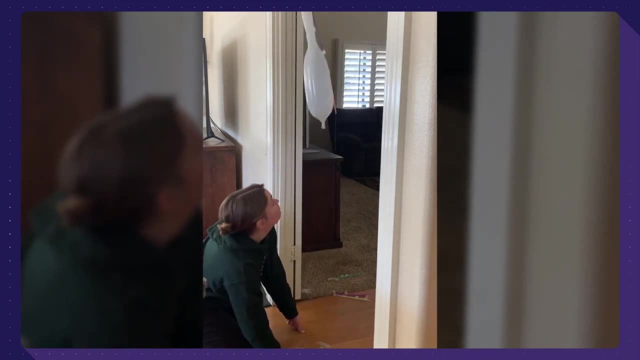 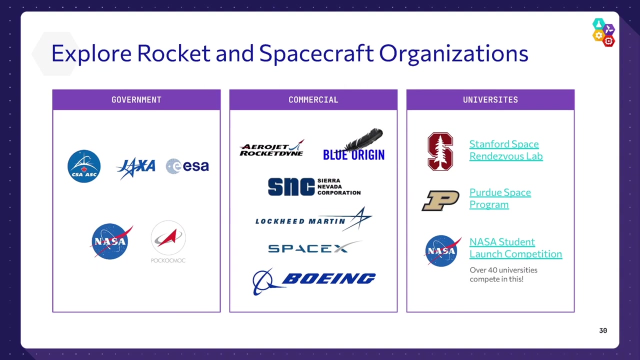 better idea. so, if you enjoyed this, we want you to continue to explore rocket and spacecraft organizations now. the government is a great place for you to explore. it's a great place for you to work. there are a lot of established government agencies from across the world that are involved in space. 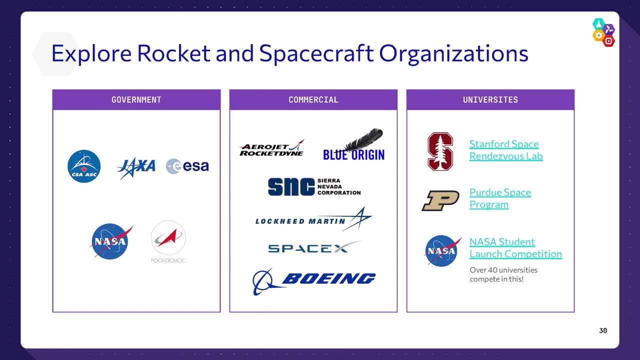 but there's also commercial entities as well: lockheed martin, northrop grumman, spacex, boeing- they're all in the space race and they're great places to work and they're working on innovative products that allow us to do some of the things like develop rockets even better and better than we've ever done before, because they're making 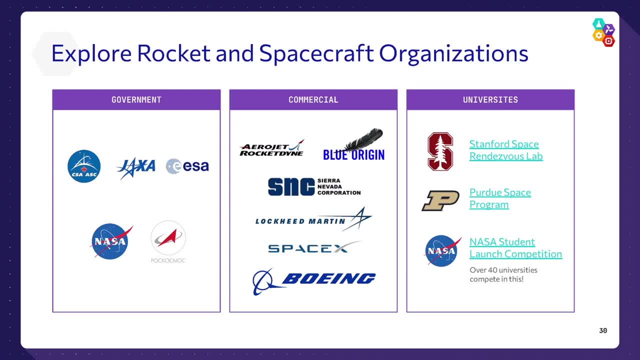 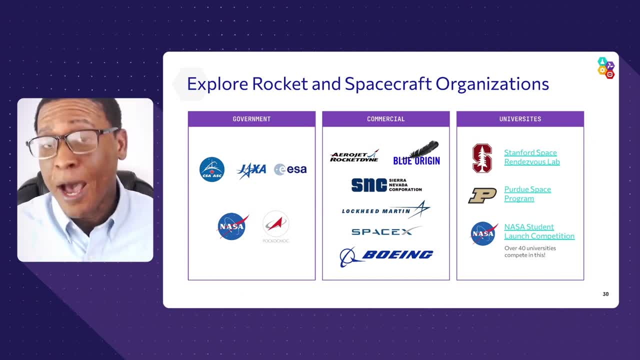 hundreds of them so they have the opportunity to really improve, and it starts really with universities. so we want you right now, if this is what you're thinking of doing, start looking at some universities now. i'm pretty biased towards purdue. i thought that was a great university. 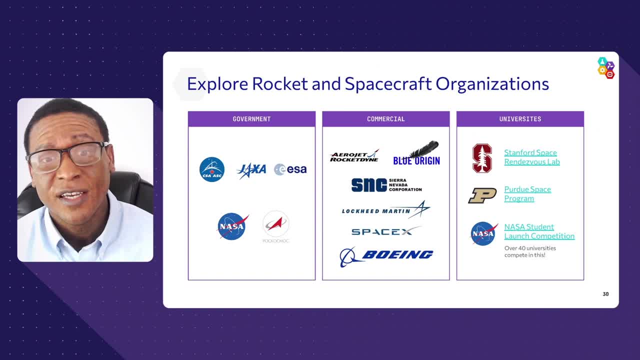 up. but stanford has a great program, university of maryland and even nasa has some different launch competitions you can get involved with both from a university and collegiate standpoint. but even while you're in high school right now, all right, hey, we're not done. i got a couple things i want. 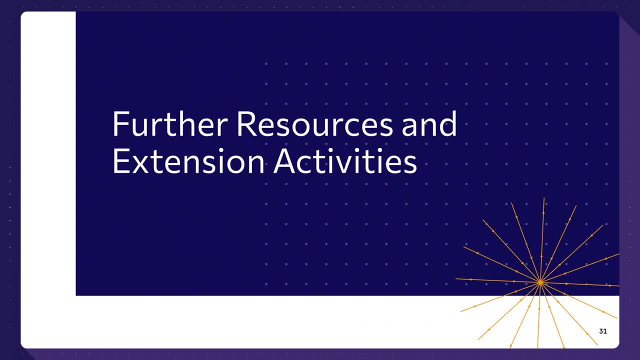 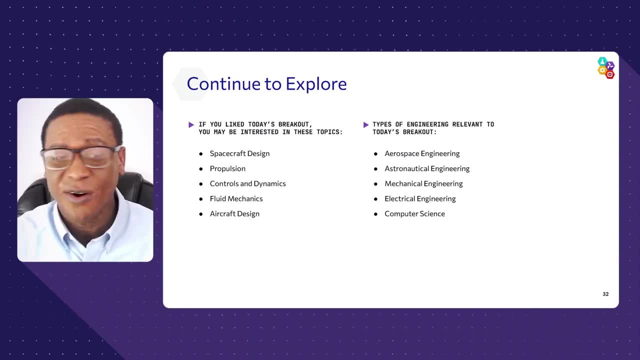 to show you some other resources, some other activities i would love for you to see. but as you continue to explore, if you enjoyed spacecraft design, if you're interested in propulsion, if you're interested in aerodynamics or fluid mechanics or aircraft design, here are some fields that you should investigate. we talked about aerospace and astronautical. 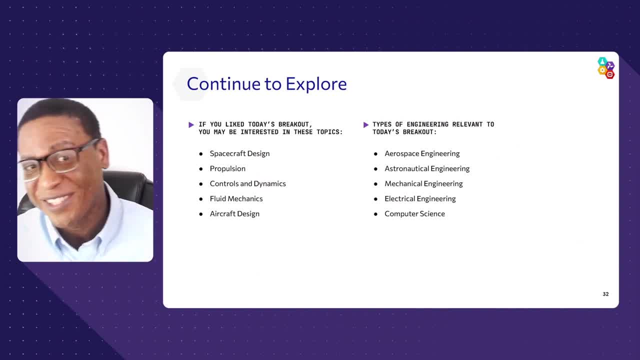 engineering. aerospace is everything in the atmosphere. astronomical engineering is everything beyond the atmosphere. but you know, none of this is possible, none of these vehicles are possible without mechanical engineering, the structure that has to be developed. how do we make sure things don't fatigue or break as we're trying to launch through this crazy gravity and crazy? 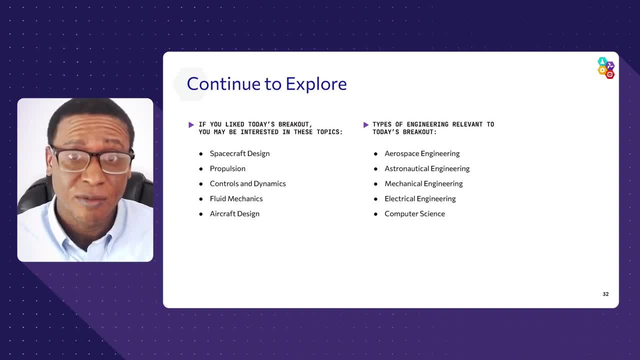 atmosphere in the space. all that's important. electrical engineering is important. i mean, space vehicles are electrical systems. they have batteries, they have solar panels, they have, um, avionics like a brain that controls everything. and then, since we talked about avionics in the brain, computer science. a lot of this stuff has to be automated, so we need software developers. 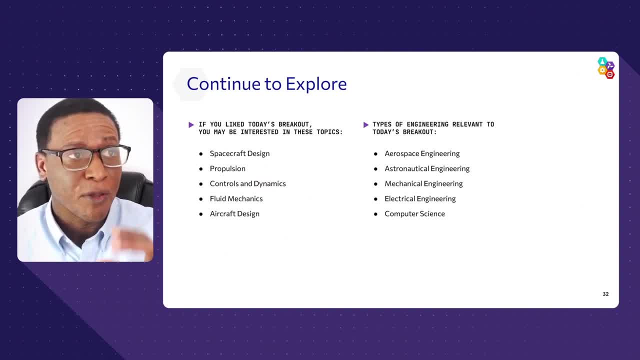 and coders to program the spacecraft so the the mars rover can perform activities all timously and not have to wait hours for a signal to come from the earth. you know, you can see, almost every single engineering field can be involved in aerospace. all right, so here's that last mission i want to talk to you about now. what if you? 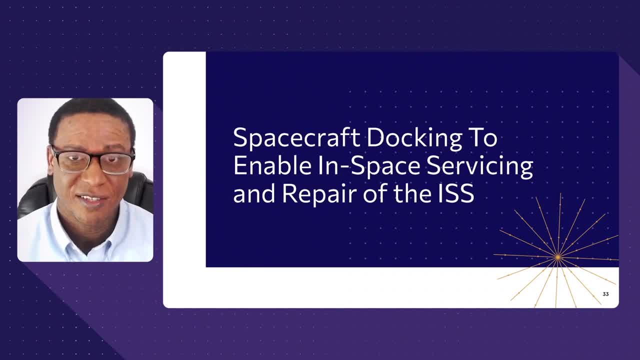 wanted to dock with the international space station. imagine you're an astronaut and you're going to get up there and you're going to be working from astronauts across the world. first, we got to get you there and that's what we're doing with this challenge number two. we 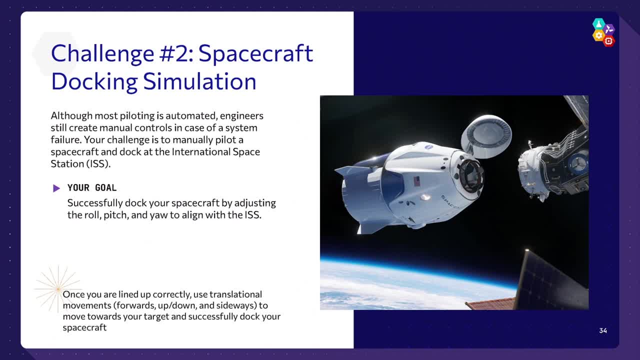 have a spacecraft docking simulation going to automate and control this capsule to navigate its way all the way to the international space station. you're going to do this with a very cool game. you're going to use some very cool controls like roll, pitch and yard. you're going to change your speeds in different directions. 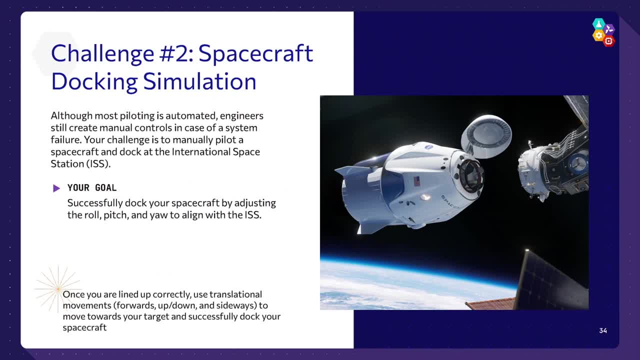 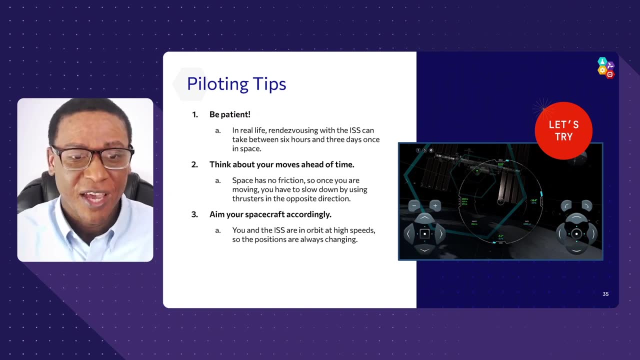 you're going to break, you know. you know, navigate through all these uh different, you know physics so that you can end up having an astronaut that rendezvous on to this capsule. so it actually looks pretty cool. it's like a cool game. you have your controls. it reminds me of playstation 5 and 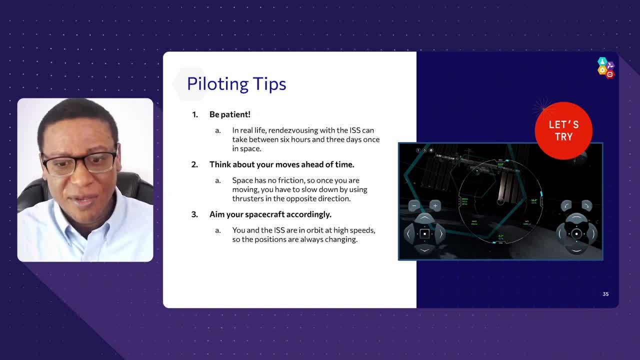 you're really changing that role, you're changing that yard, you're changing that pitch and so, ultimately, you're finally able to get there. now. it took me about 20 minutes to even get this thing working, where you know i could navigate very effectively, hey, but some of you all are gamers. 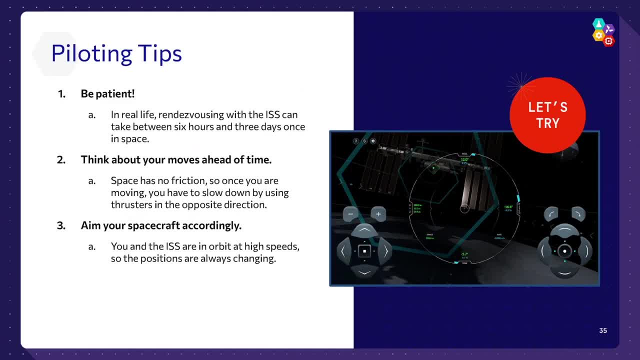 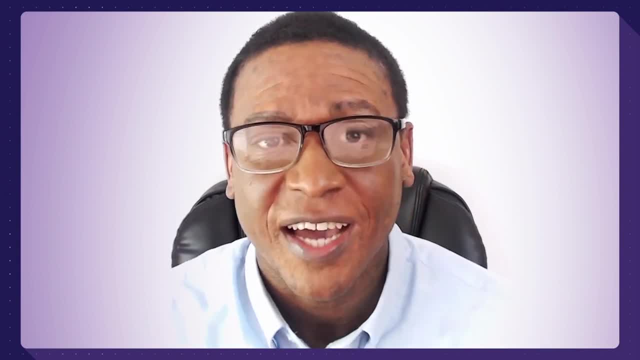 maybe you'll do it even faster. well, with that, i want to say thank you all so much. i'm so excited to see you all. i hope you enjoyed this video and i will see you guys next time. peace, xoxo. see what you all would develop. I can't wait to see these rockets launching and I can't wait to 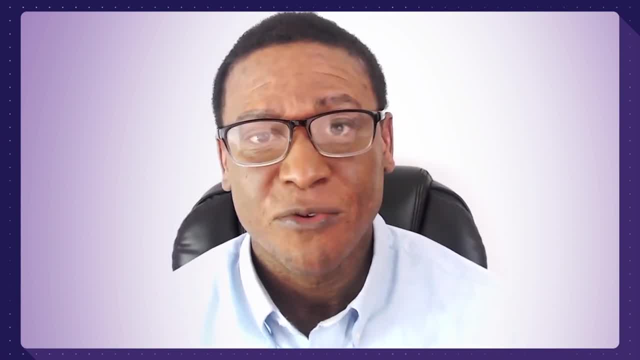 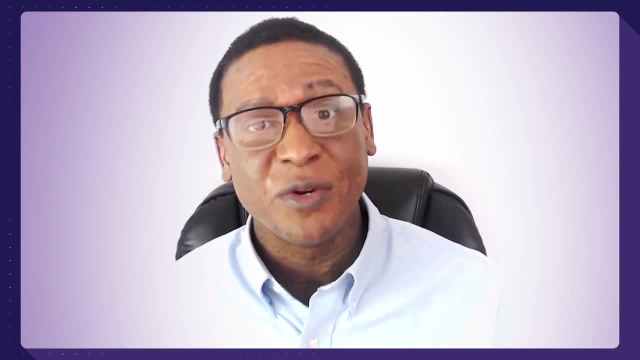 see you docking in this very, very cool docking game. So your next steps will probably be a Q&A with some of our awesome college students And then after that, you'll wrap up with maybe an engineer just like me, where we're going to talk about how great you perform in your lab, or we're 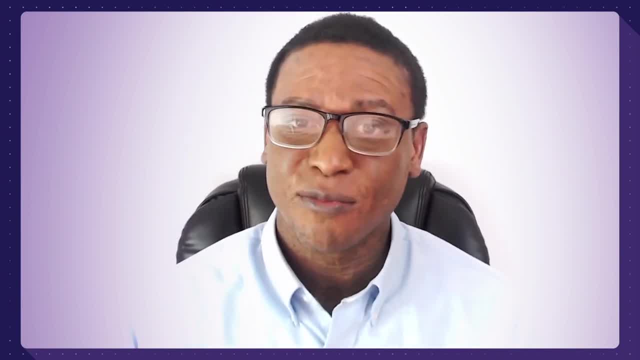 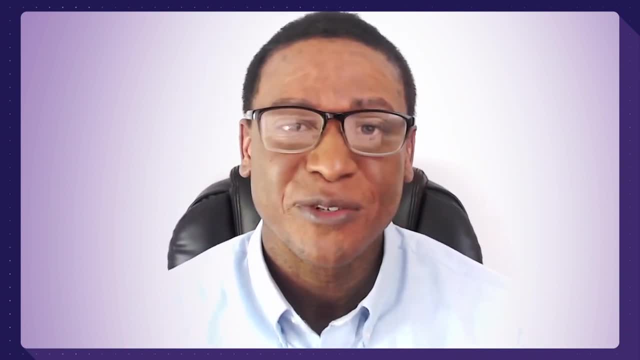 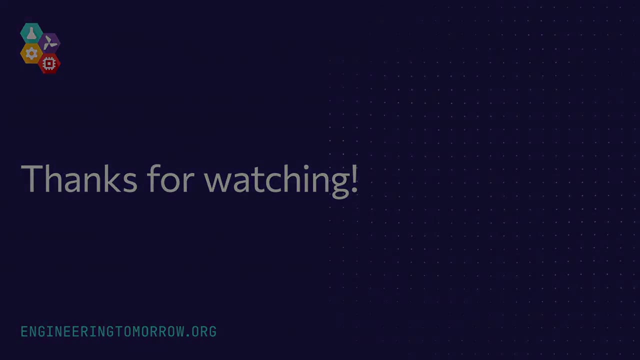 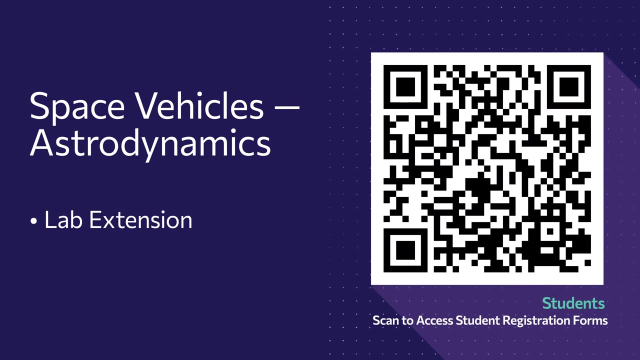 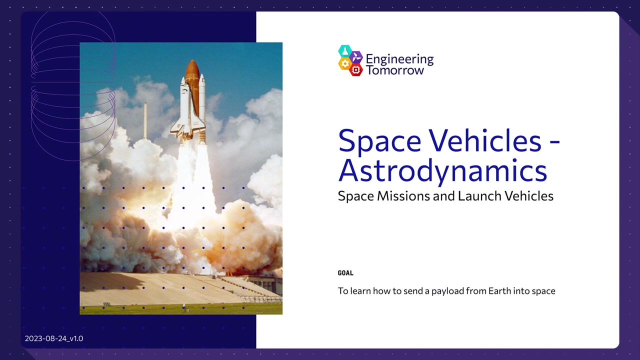 going to help you improve it real time. So with that, on behalf of Engineering Tomorrow, thank you so much. This was our Space Vehicle Rocket Design Lab, and you all are absolutely going to kill it. Have a good one. Welcome again. This is our Engineering Tomorrow Space and Astrodynamics Lab, where 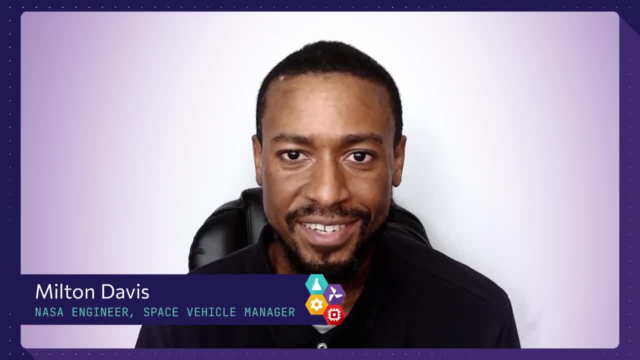 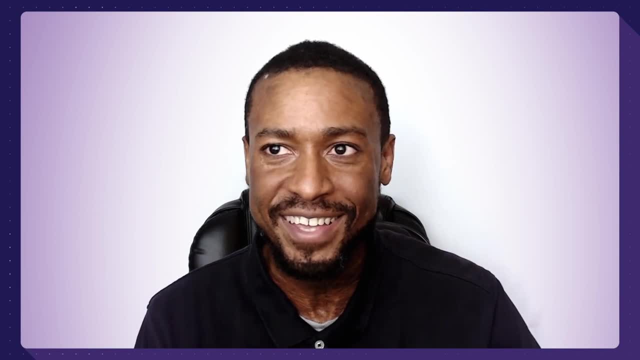 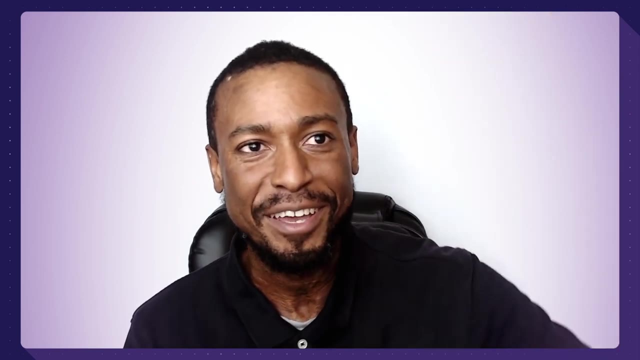 in the lab, the main lab, you all developed your own rocket. The propulsion was a balloon and your goal was to ensure that rocket not only could elevate and rise beyond the atmosphere all the way to the ceiling in your classroom right, but that it remained there. it carried a payload that's 50. 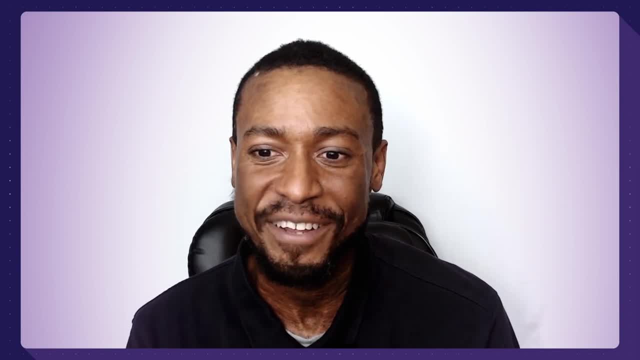 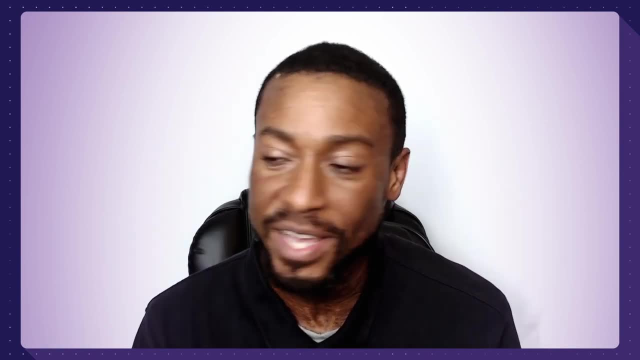 paper clips and that it came down safely. And if you've completed that or you've completed a lab similar to that in the past, you're going to have a rocket that's going to be a rocket that's going to get out of the space. So, speaking of rocket Engine, we'rely you to make the appropriate 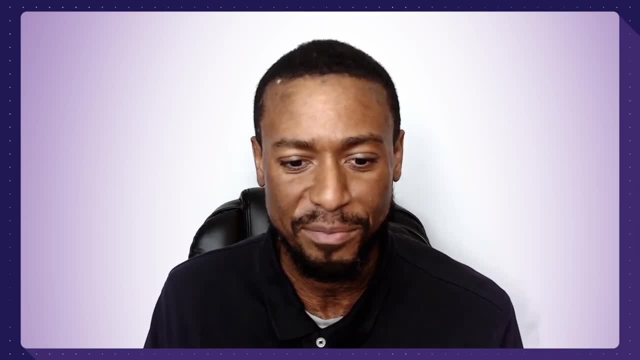 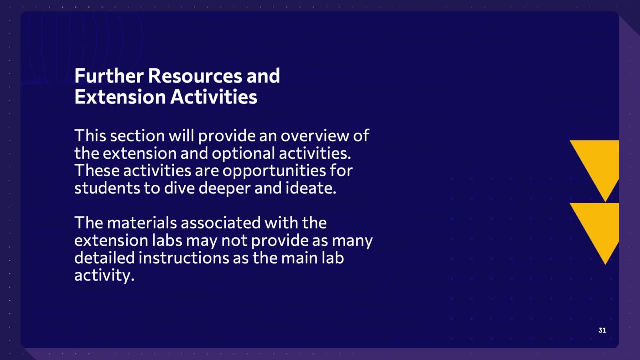 competition. today We have a great opportunity for you. We have some very nice space extensions. What's extensions? Why is that important? Extensions give you the opportunity to ideate and innovate even greater than what you've done in our base lab. Here are the extensions we have. First, 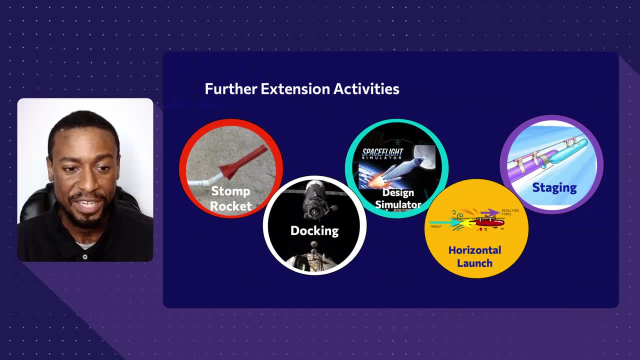 we have a couple of simulators. The design simulator allows you to build a rocket and launch it. This docking simulator allows you to simulate taking a capsule to the international space station. And then we have, you know, some physical labs as well: staging to improve your 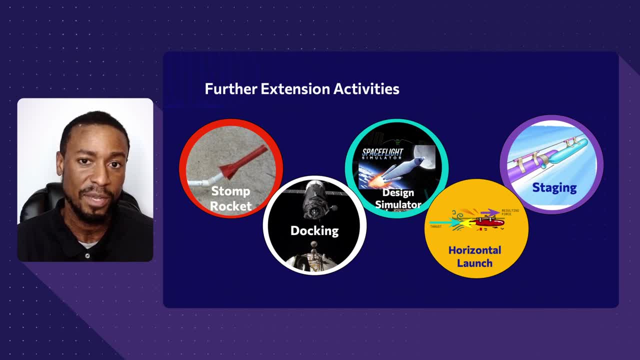 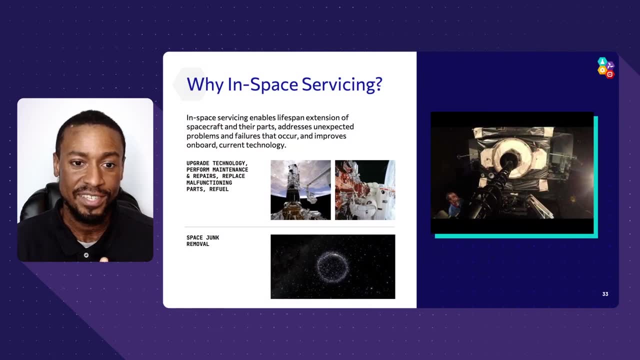 horizontal system or your vertical system, which we'll talk about in a stop rocket, okay, But for a little context. the reason that we are working through a lot of this is our goal is how do we improve satellites that are already in space? Now imagine you got a satellite in. 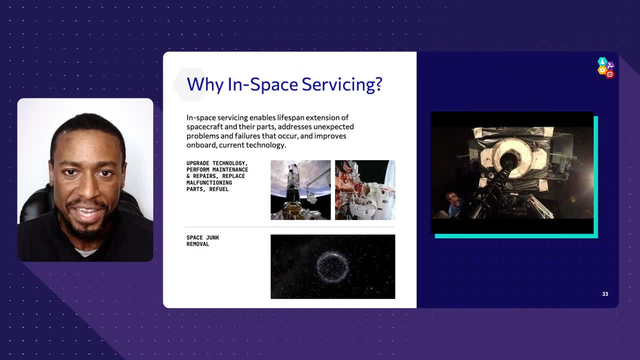 space just ran out of gas, or maybe it has a bad computer. Could we fix it? That's what in space- servicing, assembly and manufacturing- it's all about. Take a satellite that's working- you know, performing great science- and fix it by either refueling it or replacing one of its parts. 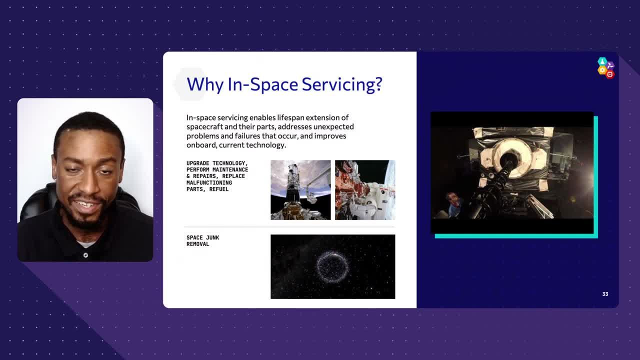 And we're doing that robotically, like you see in the image. In the past we've done that with astronauts, but we want to see if we can do this robotically and maybe in the future, autonomously. all right, So let's talk about extension number one. Extension number one is staging And with 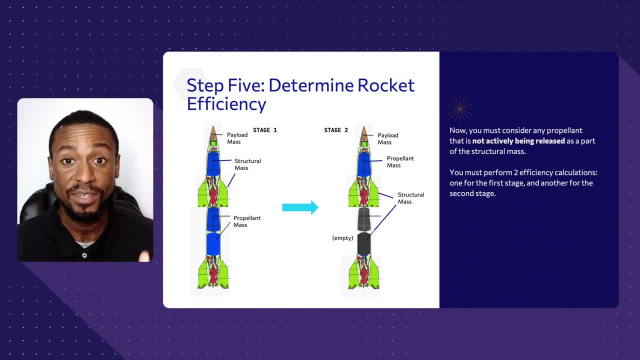 staging. you took that vertical-based rocket that you developed right, And we are going to add another balloon, another rocket system, so either you can attain a greater height or sustain height for a longer period of time, And it's exactly what we do at rockets right now. A rocket that's 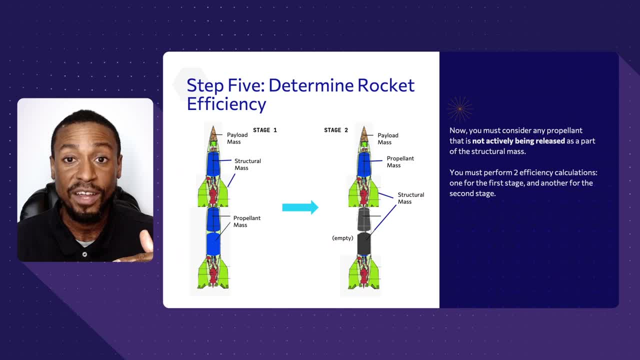 developed may have three or four stages: a stage to get it off the ground, a stage to get it further through the atmosphere, And maybe a stage that will place it in the correct orbit. right, That's staging. How do you do it? 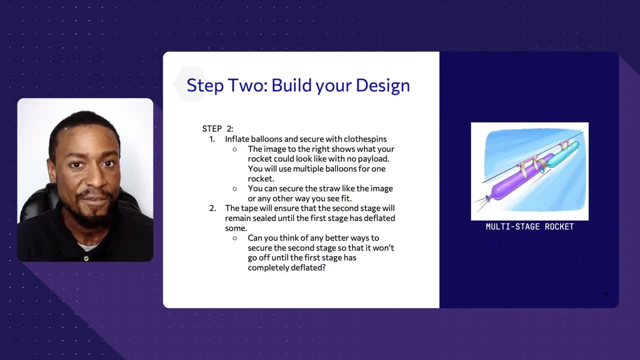 Well, you take those current rocket balloons that you have and you find a way to connect them and assemble them in a manner where you'll get most of your thrust coming from your first stage And then, after that stage has completed most of that thrust, most of that push, then the second stage will kick. 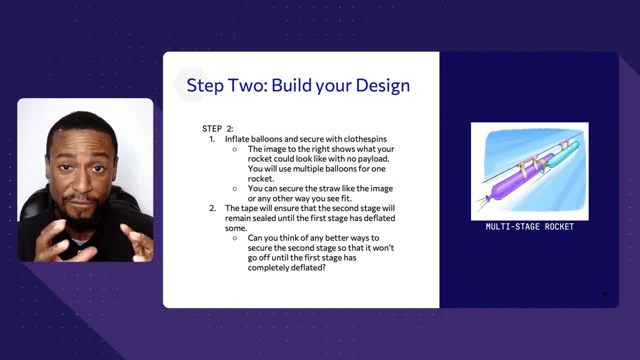 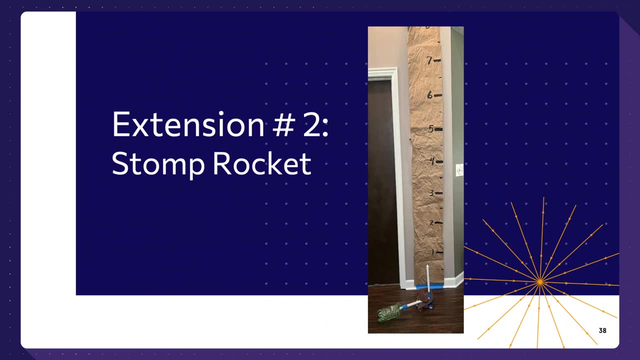 off And it'll give you the rest, And the innovation for you is to design some sort of mechanism that is going to allow you to switch between the stages. I can't wait to see what you're going to create. So that's extension one. Extension two is the stomp rocket, And I have to give a shout out to: 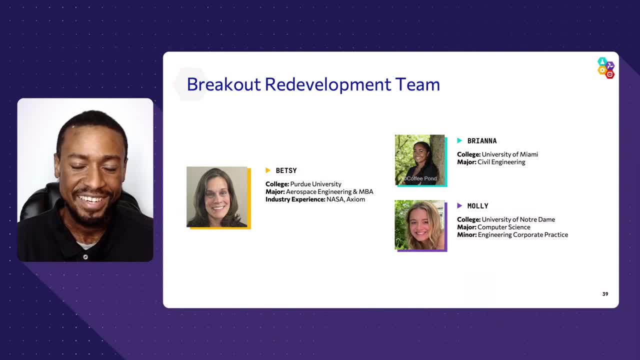 the team, Betsy, Brianna and Molly, for putting this together. Hopefully this is something that you'll see, that you can take advantage of a rocket and develop it and get a lot of benefit out of it- A lot of speed and a lot of force, and maybe even rocket launch it outside. So here are your. 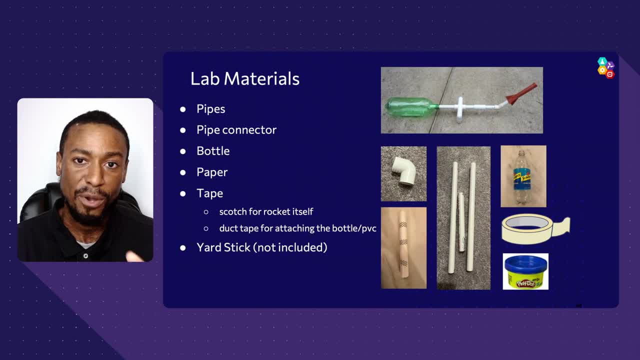 materials. It's a little different. We're not using the balloons. Our propulsion is going to come from this bottle that you're going to place some pressure against And you're going to use some PVC pipe and tubing. bring it all together and launch this at different angles, different. 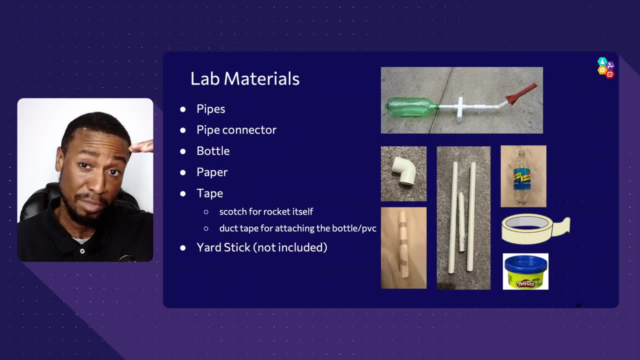 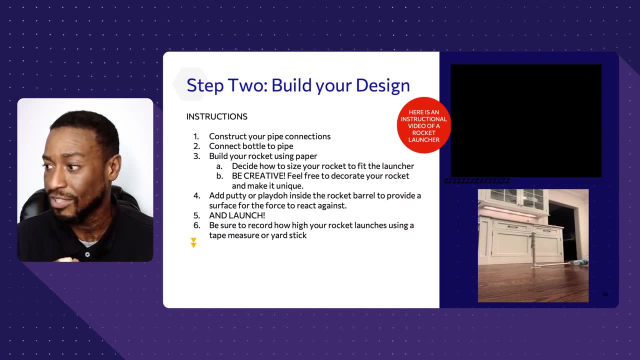 trajectories and see if you can assess not just the maximum height, but can you assess the velocity, Can you assess the acceleration. So here's a kind of sample of some of the instructions, But let me show you a video as well of how we're doing this. an example: Here's a nice 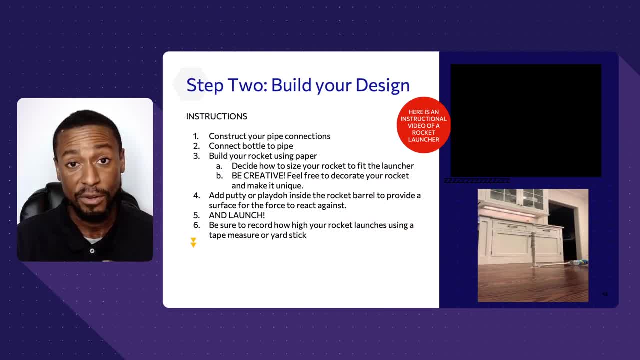 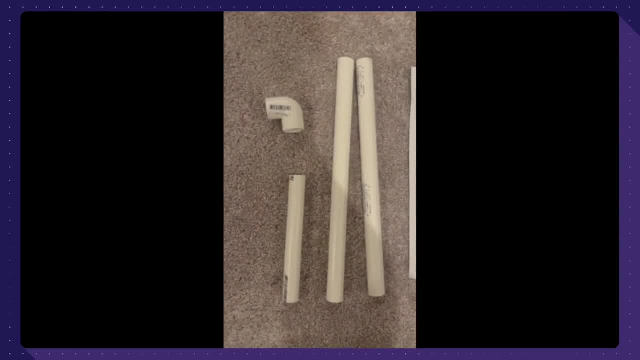 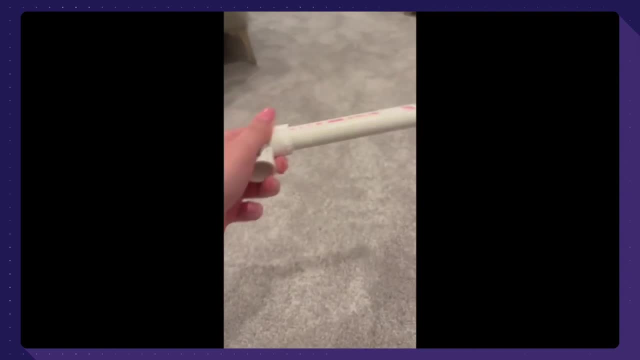 construction video that you can see that works through how to build it. In order to complete this challenge, the materials you'll need is a bottle PVC plastic pipes, a piece of paper and some tape. The first step is to connect your PVC pipes in order to create your launcher. 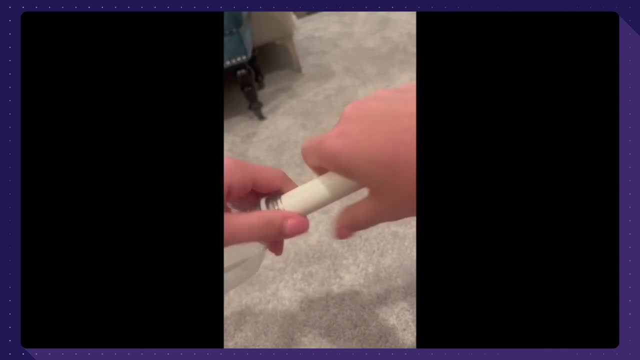 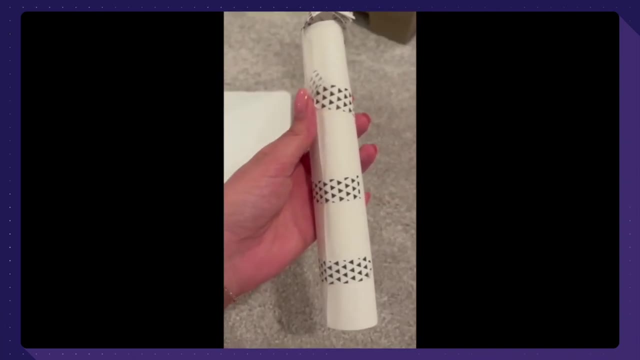 Then connect your plastic bottle that will be used to build the launcher. Then connect your plastic bottle that will be used as a power source for your rocket. Next, I created my rocket design with some paper and some tape. But be creative. there's so many designs you can do. 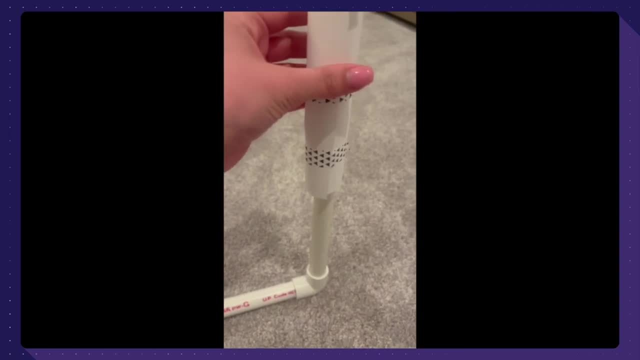 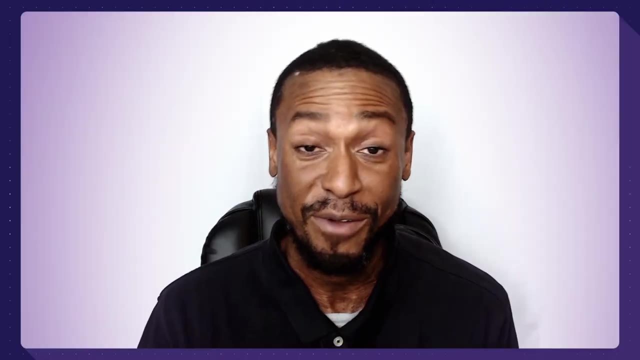 Next, I stuffed my rocket with some paper so that I could balance on my launcher, And that's it. Then your design is complete. So that was the instructional video on how to build it. This next video will teach us talk about how to launch it. 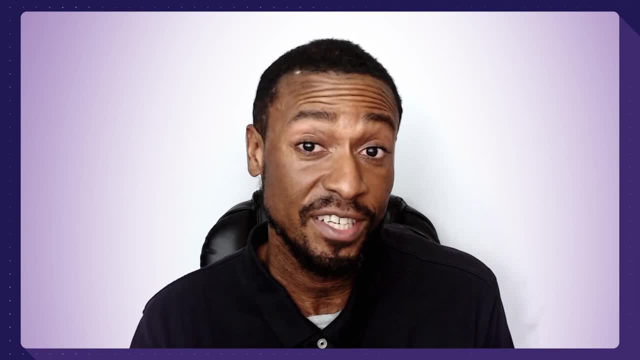 And just remember: this video shows us launching in a room. It's safer to be able to start it off. So here's a video to teach us how to launch it. And just remember: this video shows us launching in a room. It's safer to be able to start it off. 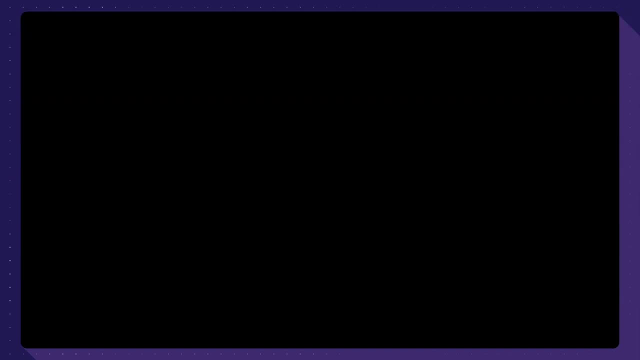 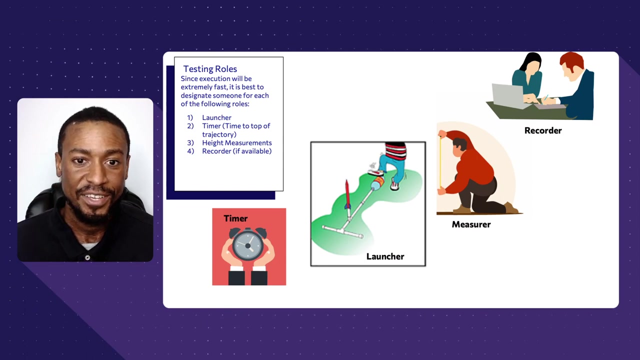 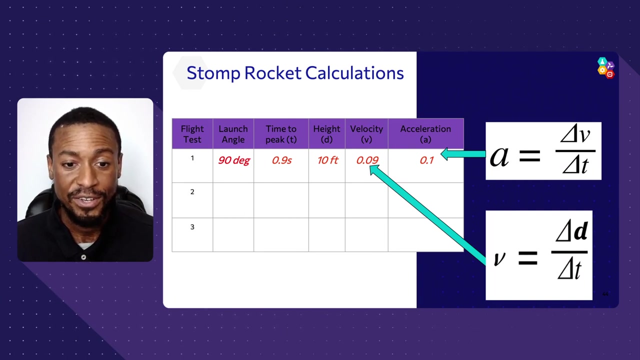 to launch outside. so that's what we recommend all right, now that you have launched the system, you can perform some calculations, as we talked about. if you're able to somehow estimate the height, you can also um calculate the velocity by using um, based on your launch angle and in. 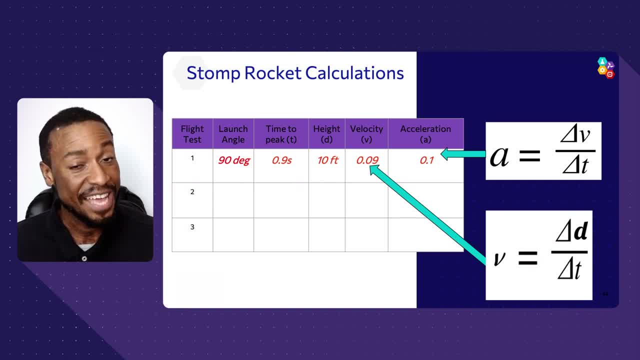 your time, we can calculate velocity. and if you- if you haven't heard this before- if you take the change in distance over the change of time, you get velocity. and then you take the change in velocity over your change in time and that is how we get acceleration. 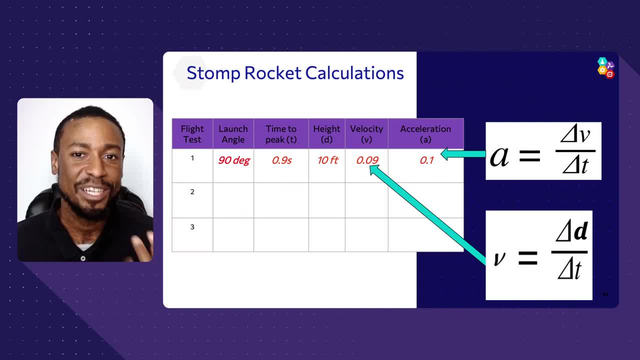 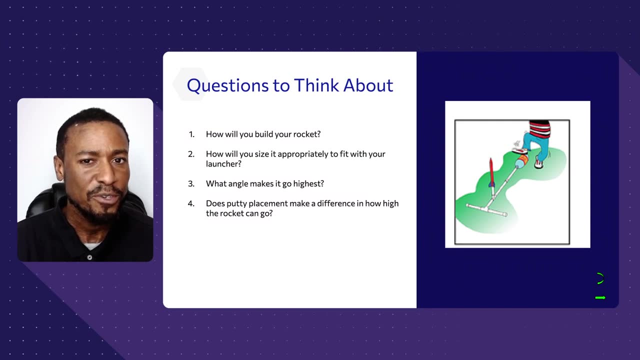 and if you didn't obtain the height or the acceleration or the velocity that you desire? that's where you have an opportunity to improve as you're developing the design. here's some things to think about. how would you build your rocket? how would you improve it? what angle truly gives you the best results from that rocket? that's. 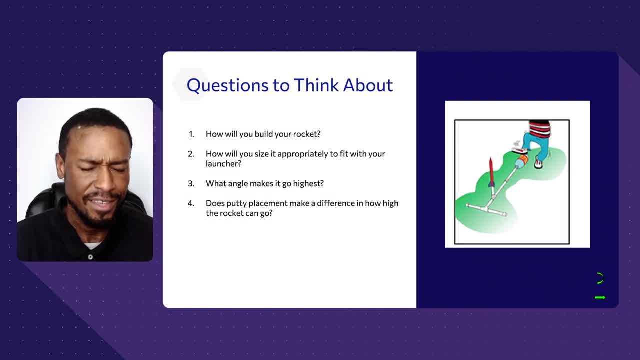 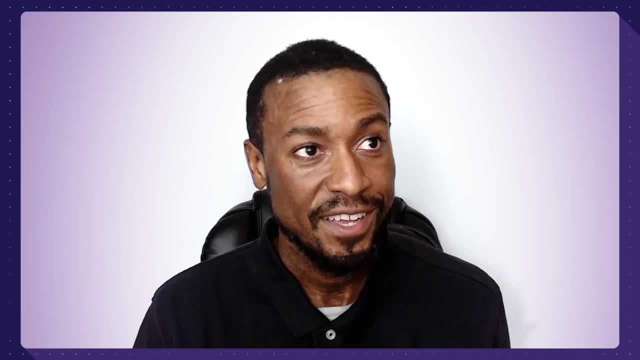 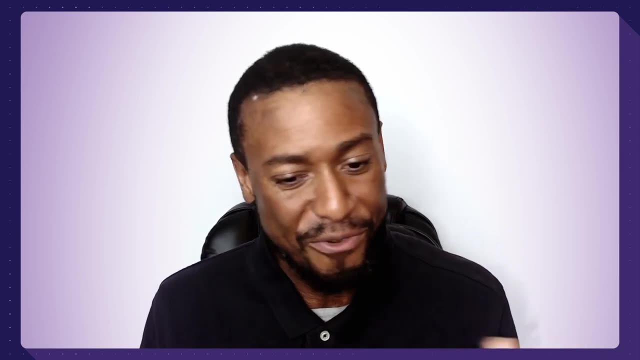 that's what we, as engineers in the space field, think about a lot, that that trajectory that's going to get us into the right orbit. great well, you finished extension 2 and now that you've developed this new super fast rocket, extension 3 is all about. what are we taking into space? 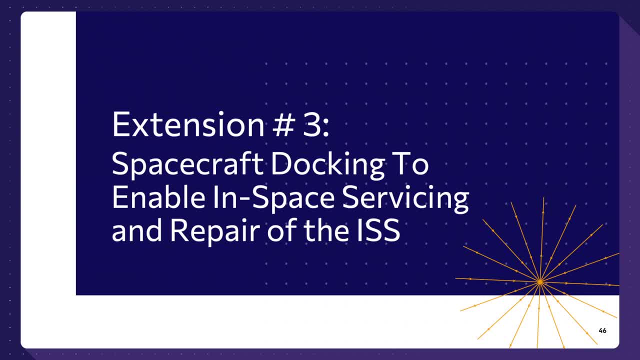 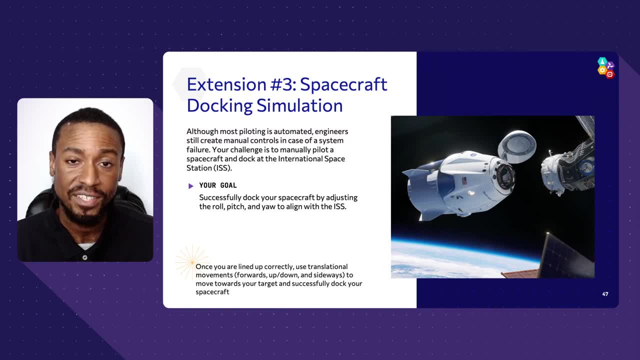 your rockets space. now what are we going to do? well, here's a great idea. this is what spacex does. they have capsules that they will send to the international space station. that may be carrying cargo or food or astronauts to the iss, and that's what you're going to simulate. spacex developed a really nice 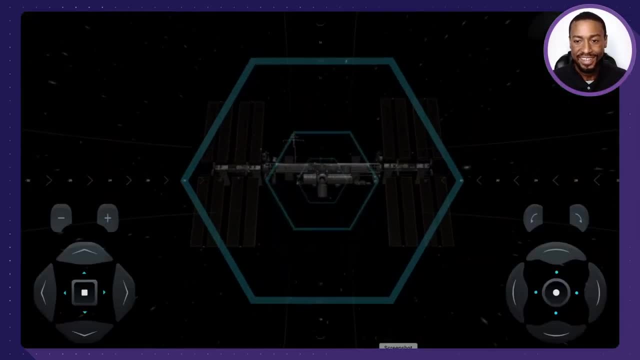 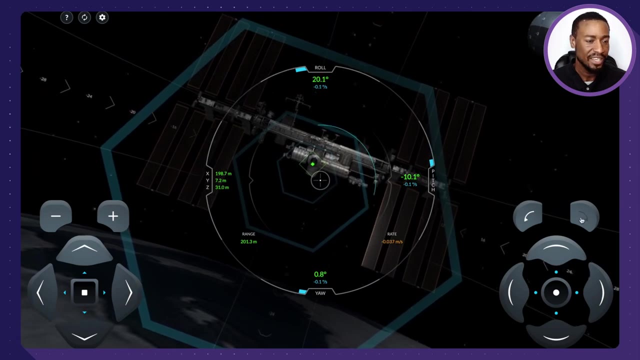 simulator that allows you to kind of simulate or emulate you being the one in control to take this capsule from its destination to the space station, and then you're going to be able to take it to the destination where it is been removed from the rocket, to the actual iss right, and to do that 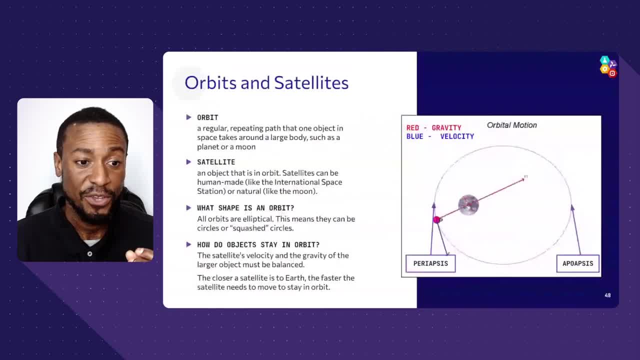 you got to know a little bit about orbits, right? you? you had to placed that rocket, had to place that capsule in the correct orbit. the orbit is ultimately the path that your, that your satellite or space field- cool- is navigating. your satellite is your instrument, or, in this, 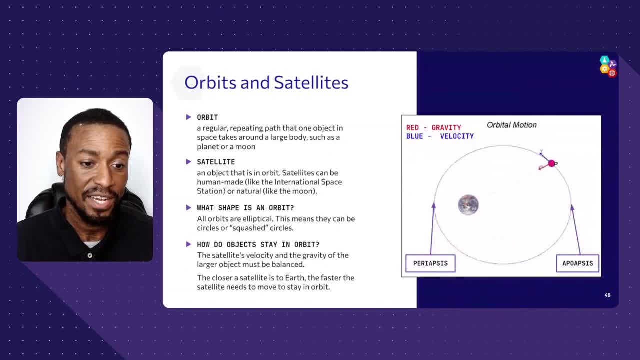 case this capsule, it could be some cargo for the astronauts. the orbit is going to be a little bit different. it's going to be a little bit more elliptical. right, it's not perfectly, it's not really circular, because there's a lot of different planets out there that are 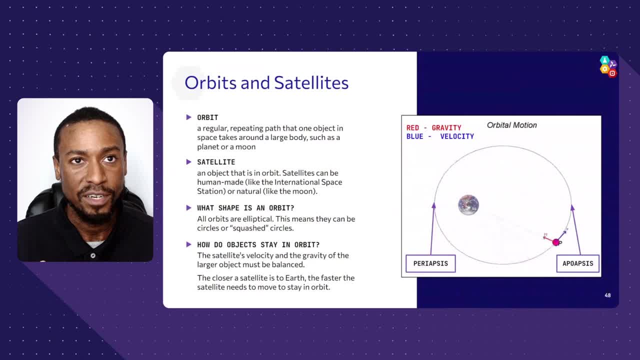 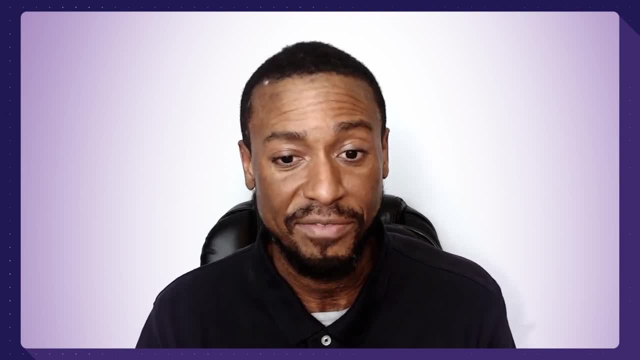 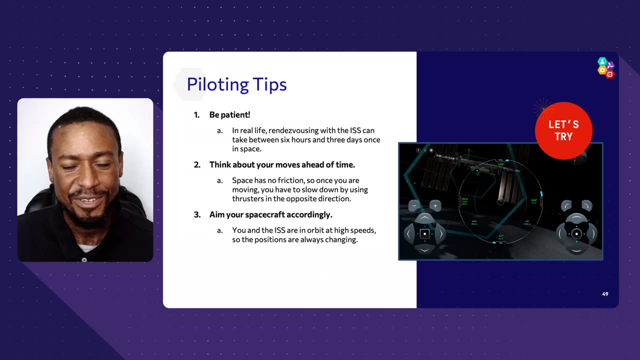 pulling and tugging on our on these different objects in order to have a optimized trajectory just based on gravity, and then you know they stay in orbit one because of that tug, because of that pulling, that's happening, okay, so now you know a little bit about orbits. you got to control this. 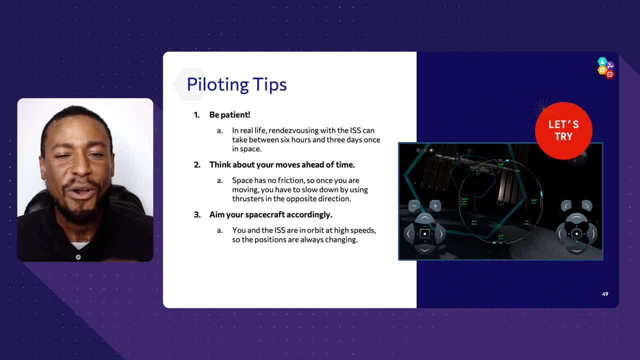 this capsule. so how do we pilot? how do we do this? let me give you a couple piloting tips. as always, be patient. this is not easy, even in a simulation, and it shouldn't be, because we want simulations to prepare us for what's going to happen in reality. so be patient, you know really. 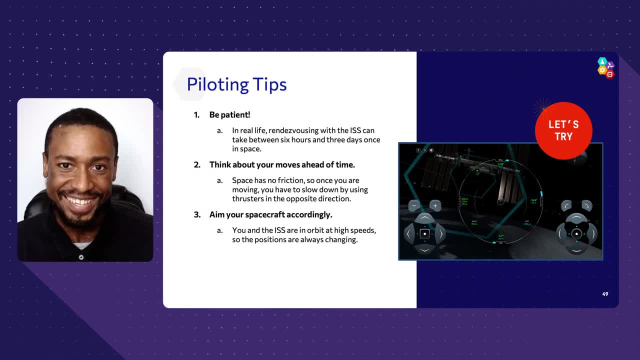 just like with a video game kind of map out your strategy ahead of time. you know how how much, how many times, how much effort are you going to apply to moving left and right? are you going to, you know? think about that. are you going to take it slow? are you going to do it right? are you going to do it? 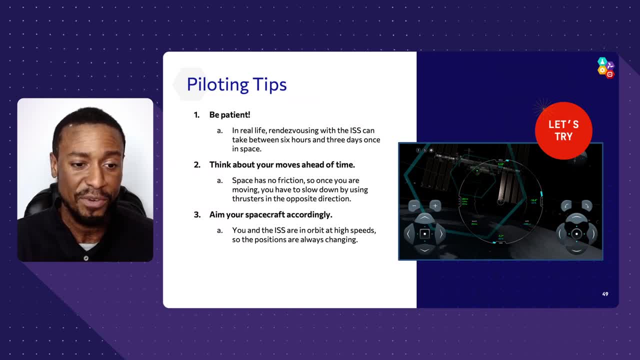 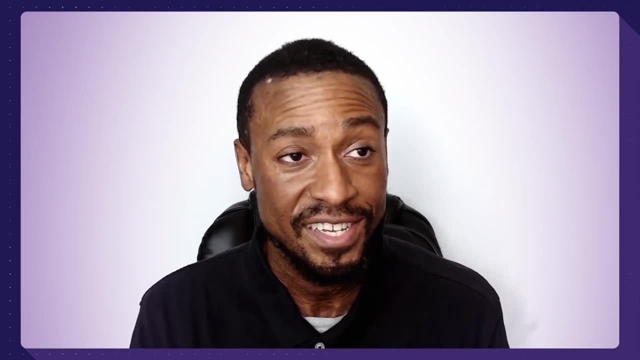 think about how you're going to rotate. you know your translation, your rotation are going to be very important, um, and then just aim your spacecraft accordingly. so i think i think you're going to really enjoy this. the first time it took me about 40 minutes, but what we really want to see, 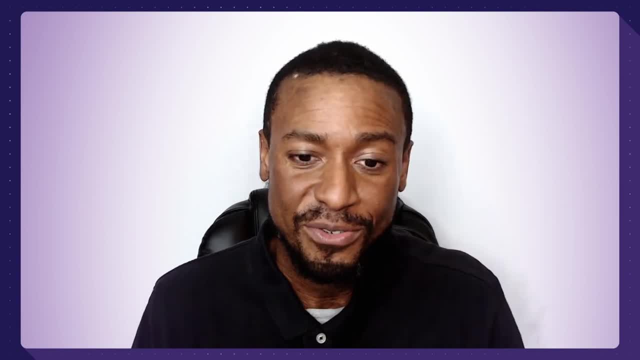 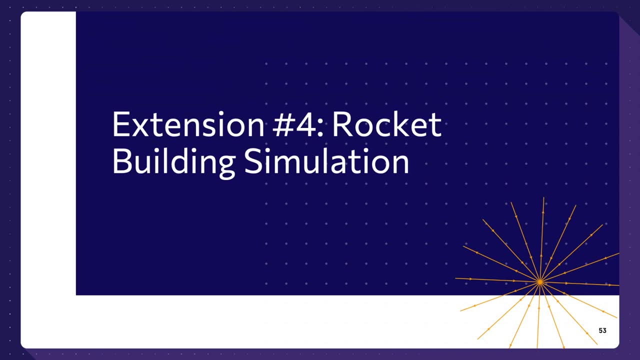 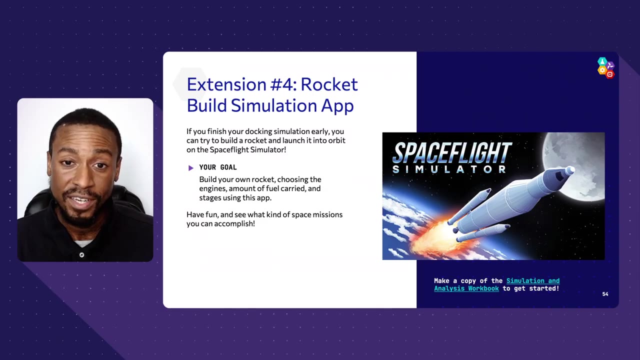 is: how quickly can you navigate this capsule to the space station? so that's our third extension. now, extension number four is another simulation. this is where you'll build an entire rocket and, unlike that we gave you, with balloons, you get to build something that looks more like a true rocket. 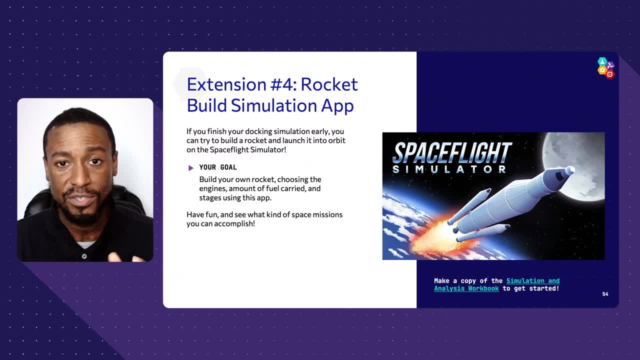 you choose all of the different systems. you know. you get to choose the structure, you get to choose the number of rockets, the type of rocket fuel, the stages, ultimately, to build this rocket and launch it. very, very nice tool and if you're interested in aerospace, this gives you more. 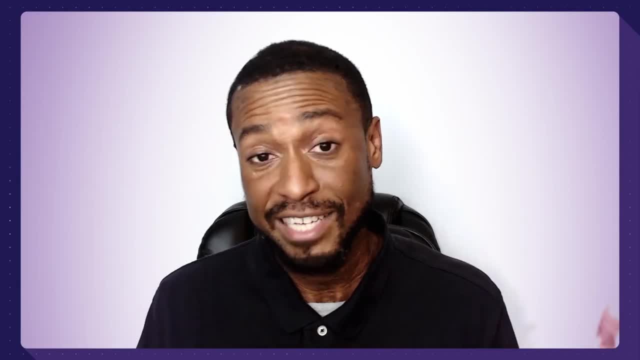 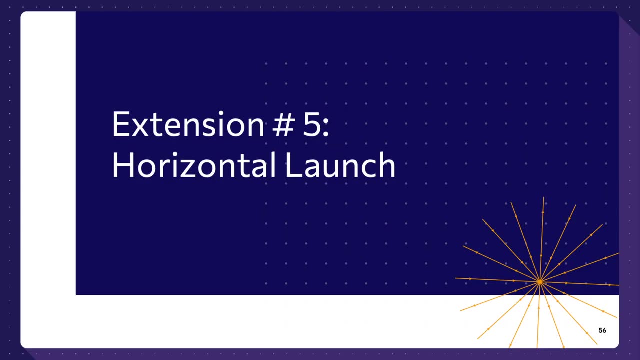 insight into the challenges and the innovations and, last but not least, very, very fun and challenging extension. take what you learned with your vertical launch and even the stop rocket, and you're kind of applying it all in one activity, in one extension that we're calling the horizontal. 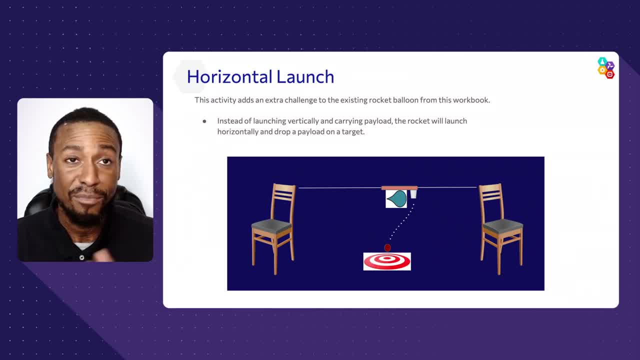 launch. so now, let's say you're taking this spacecraft to mars and maybe you're dropping the rover on mars, or maybe this is the da vinci mission. you're going to venus and you're dropping a capsule through that environment to investigate its environment, investigate its origins.